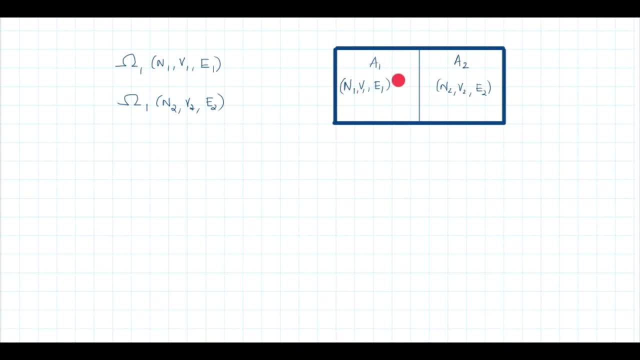 the volume of the two systems remains constant. the number of particles in the two systems will remain constant. Only energy can vary. By inserting a conducting wall, I made transfer of energy possible. The energy of the system is still a constant. Total energy won't vary. Its the sum of e1 has. 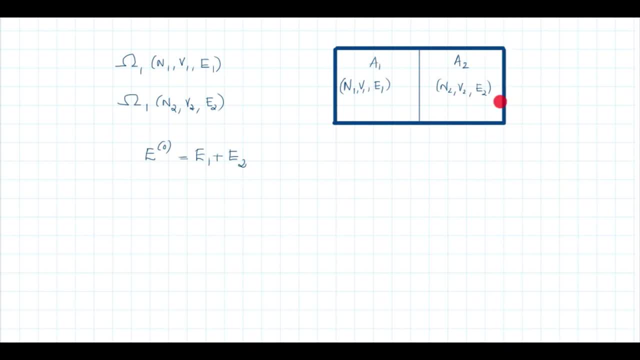 been changed because all the outer walls are still non-conducting. These are non-conductive walls that burn the energy, So only the separation from the center provides the energy exchange, But the energy of the individual systems varies and the maximum of the total energy will be constant, While 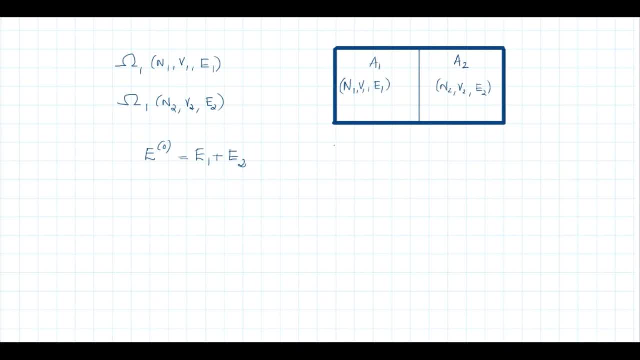 e zero is the energy of the total parts, current heart, earth and earth, and all the negative energy out of e digital area combined system. I will call that system as A naught, which is actually this combination: A1, A2.. This is the combined system. This is the combined system Now. 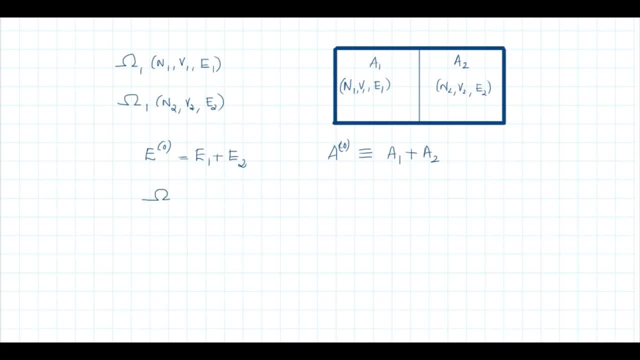 what is the number of microstates of the combined system? What is the number of microstates of the combined system? Is it omega 1 plus omega 2, or is it omega 1 omega 2? Which one will be correct? We will check that. Suppose there are four microstates possible in the first system. 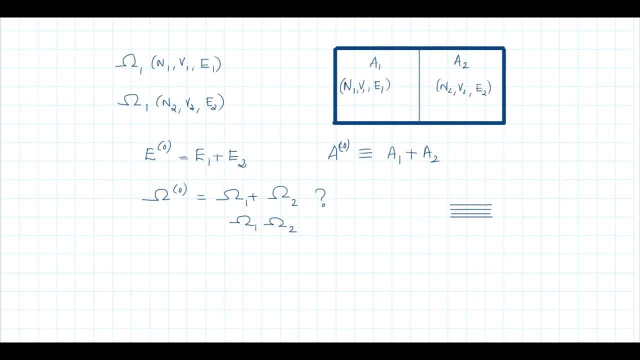 Suppose the number of microstates is 4 for the first system and let the number of microstates allowed proceed For the second system is 3.. For the first system there are four microstates. For second system there are three microstates. Then for the combined system, how many microstates are possible? 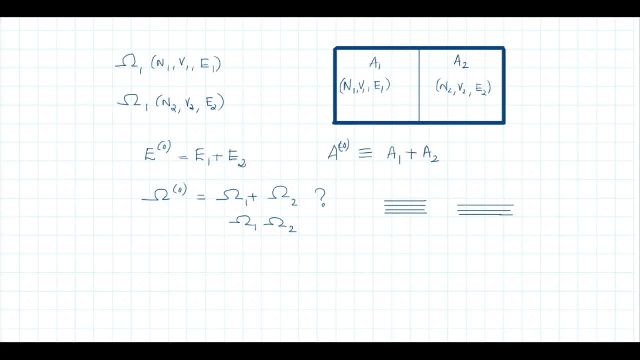 For the combined system. how many microstates are possible? When the system 1 takes this microstate 1, system 2 can take this one or this one or this one. So the combined system can be one of these microstates. It can be 11 states or it can be 12 states. it can be 3 states. 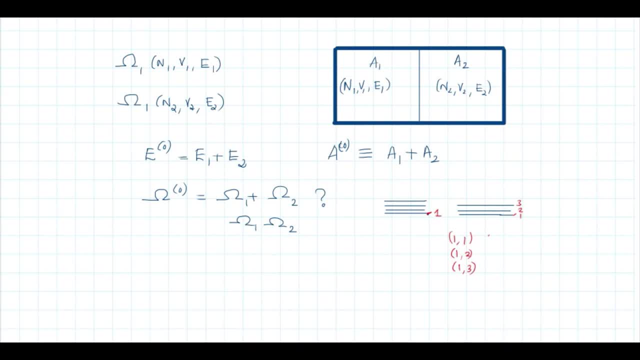 In the first system, the microstate with one is 다니ble. This means four microstates are possible For this one. you can take three. When this is one, 1,, 2 or 3 will come to this one. 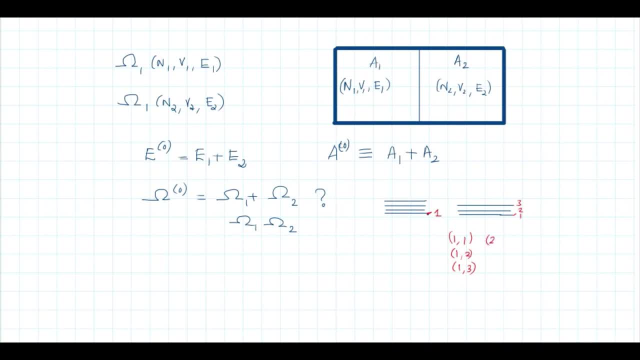 Accordingly, one will get three as per the combined system. Similarly, in the first system, when the second microstate occupies, then the second. for this system may take 1,, 2 or 3.. Yeah, Like that there will be 12. there will be 12 possible microstates for the combined system. that means, if the number of 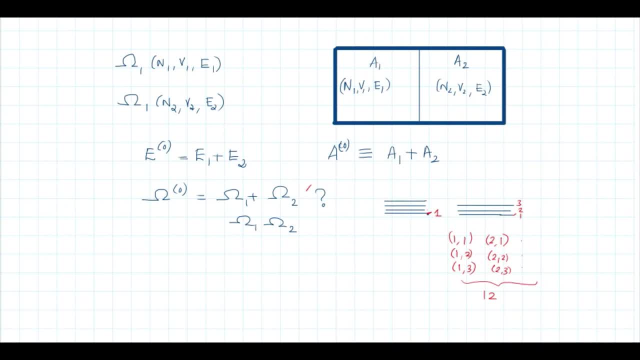 microstates of first system is omega 1 and number of microstates of second system is omega 2, then the right answer is omega 1- omega 2, so the number of microstates of combined system will be the product of omega 1, which is a function of e1, and omega 2, which is a function of it. 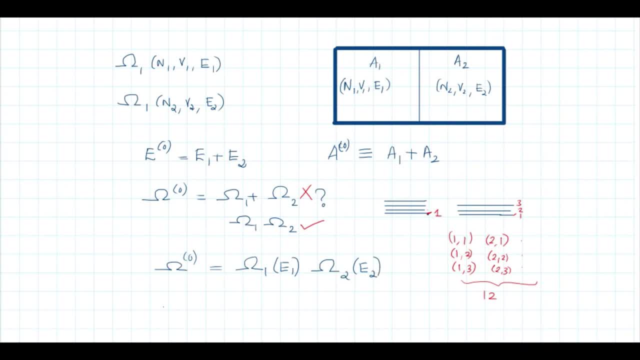 i can write this omega 0 as omega 1, e1 into omega 2- e2. but i can write omega 1- e1 into omega 2, which is actually e2. is actually e naught minus e1- e2. i can write it as e naught minus e1. 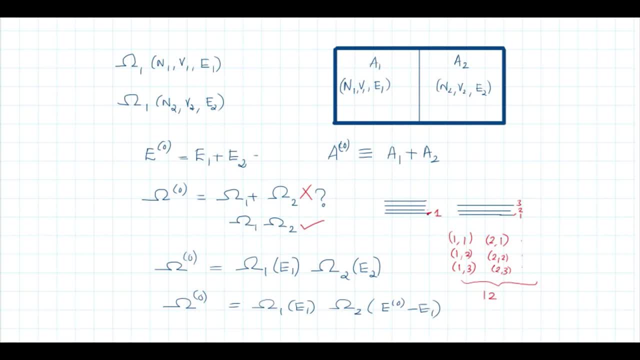 but e naught is a constant, the total energy is a constant. that means the right hand side, whole right hand side, is a function of e1, so i can write: omega 0 is a function of e1 alone. omega 0 combined, the system, is a function of e1, so i can write: omega 0 is a function of e1 alone. 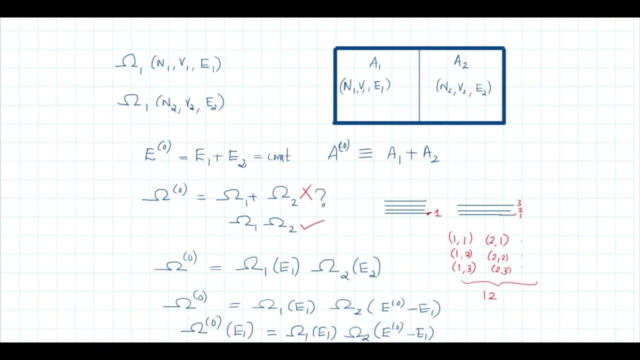 So this very first system and then this second system. it no problem that it express the energy at different time. no problem, this one will take an e2 and it will not in the same time. but what i said is that, when it comes to certain energy, a total number of microstates can be. 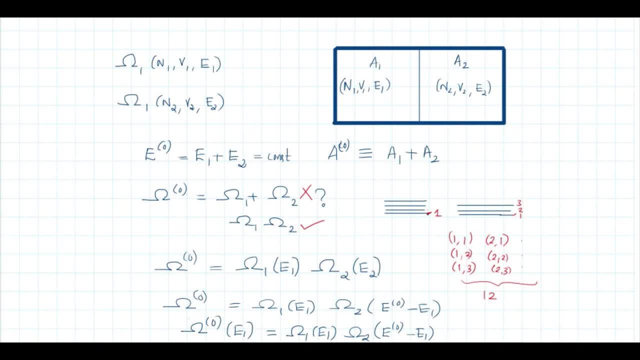 vary. If this e1 was, then it will vary the number of microstates of e1. result: it would be E2 and will vary. then this partition will conduct and then the energy will vary. that is why we said that E1 and E2 can vary. anytime it will vary, but our equation wants to be chequered. 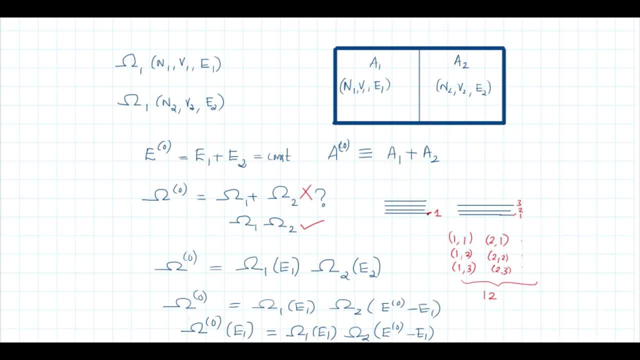 杰, energy transfer will take place When the system will achieve a new state of equilibrium, When this combined system will achieve a new state of equilibrium. When will this new state of equilibrium be achieved? Answer is: the new state of equilibrium is the one for which this. 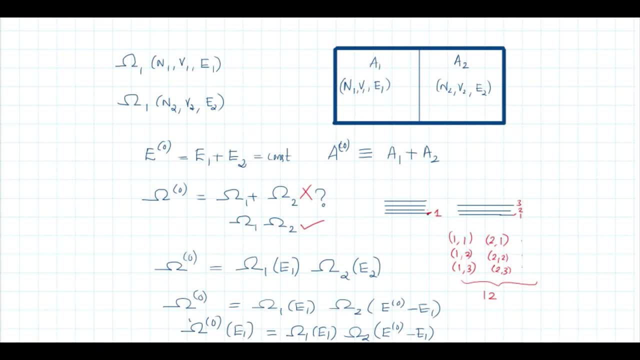 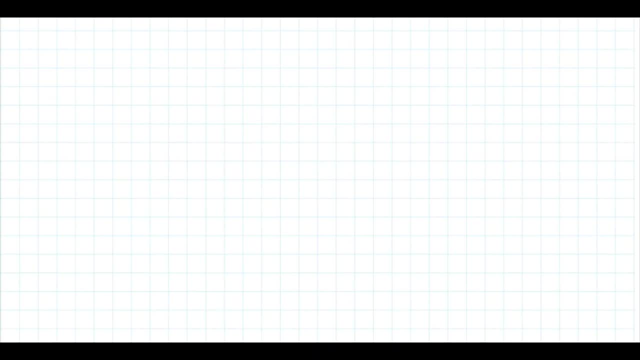 omega 0 is maximum. This omega 0,, this total number of microstates of the combined system, maximum energy E1, will be used to achieve a new state of equilibrium. Why It is so that the equilibrium state is the one with maximum number of microstates, The maximum. 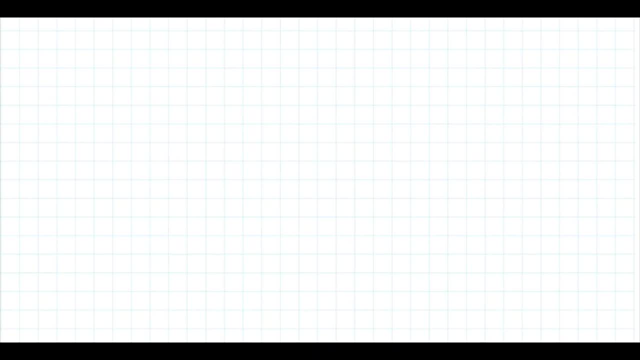 number of microstates is the reason for saying equilibrium state. Let us see In the last class- I explained an example- There are four particles, distinguishable particles. There are four single particle energy levels in the system. One is with energy 0, the other one is with energy epsilon. then 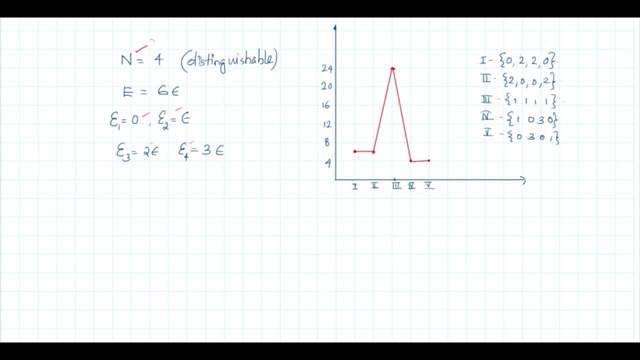 with 2 epsilon. with 3 epsilon, Four possible single particle energy levels and four particles. If we make a constraint, total energy should be 6 epsilon. Total energy should be 6 epsilon. That defines a macrostate. Total number of particles is 4. Total energy: 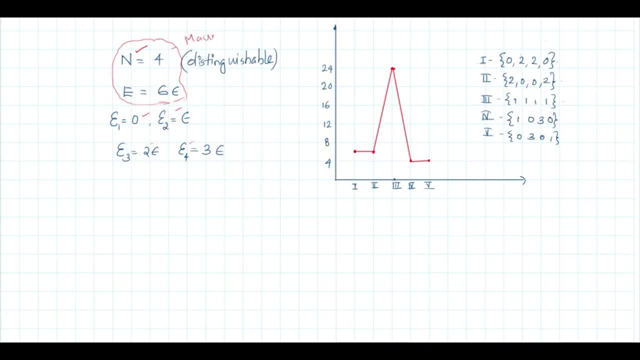 is 6 epsilon. This defines a macrostate. This defines a macrostate. Then we can see that there are five possible distributions. There are five possible distributions. The first one is: the first one is 0, 2, 2, 0. What is this distribution? You have four energy levels. 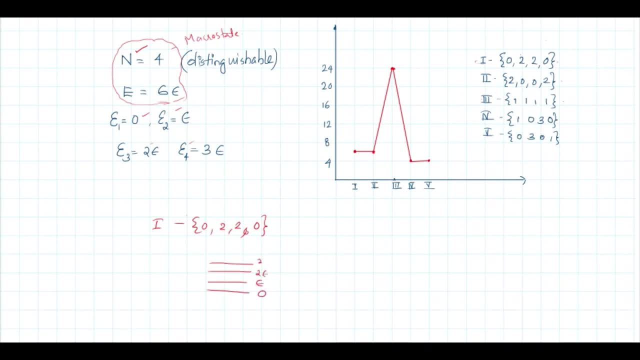 one with energy 0, the other with epsilon, the other with 2 epsilon, the other with 3 epsilon. Two particles Say, A and B, is in this state with epsilon energy and C and D the other two particles is in this state with energy, 2 epsilon. Total energy will be 2 epsilon plus 2 epsilon plus. 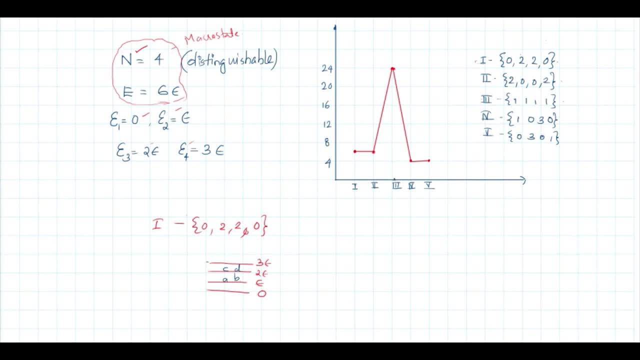 epsilon plus epsilon, Total energy will be 6 epsilon, Total number of particles is 4.. So for this particular macrostate, one of the distribution is this one. In this distribution itself we have different possibilities. We have different possibilities. 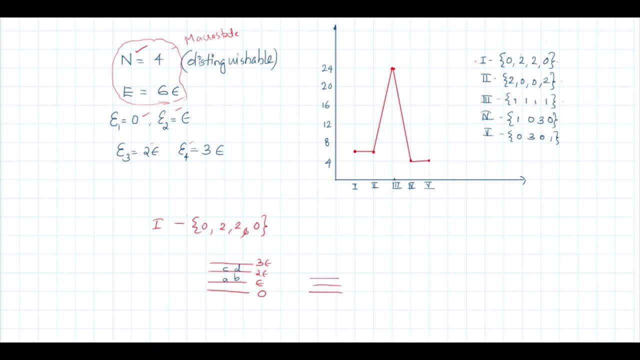 I will write this. I will write one more possibility. If you have 4, you can say that A and C lies in this state and B and D lie in this state. This will also produce a total number n equal to 4 and total energy: 6 epsilon. So this is also another microstate in this distribution. 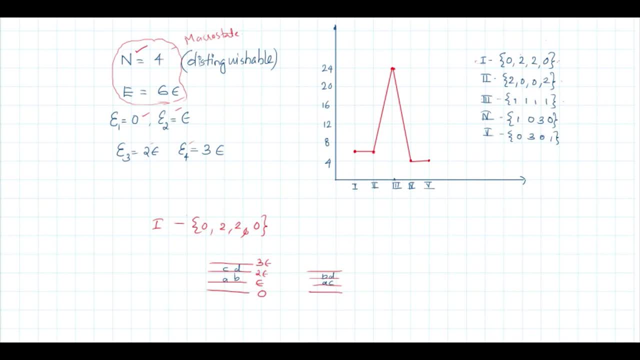 So in this distribution itself, how many particles are there? Six particles, How many particles are there? Six particles. You can write and see the different possibilities. So all this distribution can be written. You can write all the possible microstates. 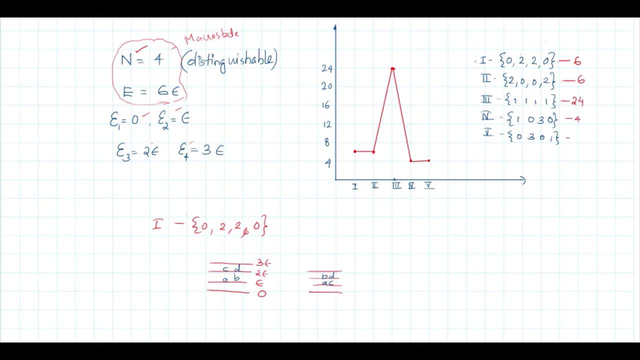 You can write and see the different possibilities. You can write and see the different possibilities. So this is the possible. These are the possible microstates in this distribution. If you see any of the previous videos, you will understand these. I have explained these. 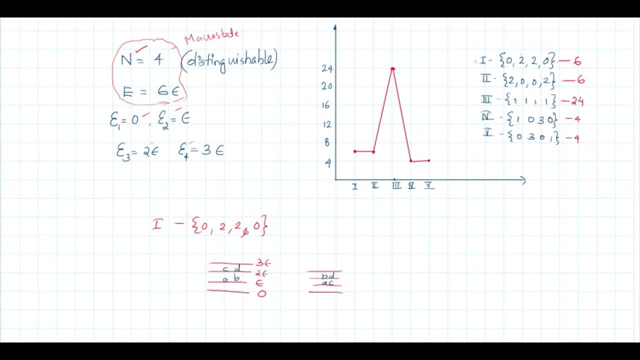 in a more detailed video. So these are the possible microstates for each distribution. So total of 44 microstates are possible for this particular microstate. Interesting fact is that the most interesting thing about this is that, if you want to plot a graph, 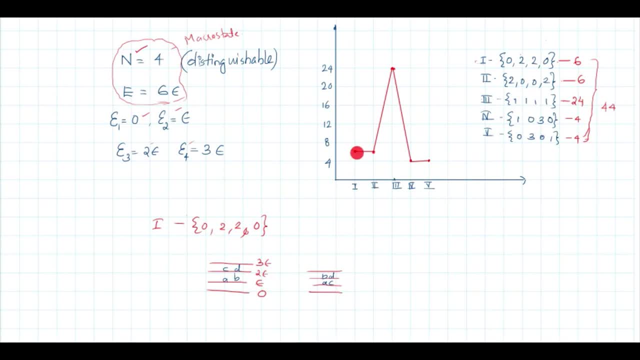 what is the distribution? Is it just a graph? Are you doing this to make a graph? Because along the x-axis number of microstates along the y-axis. So for a particular distribution the number tends to a maximum And that maximum number is very large compared to the others. 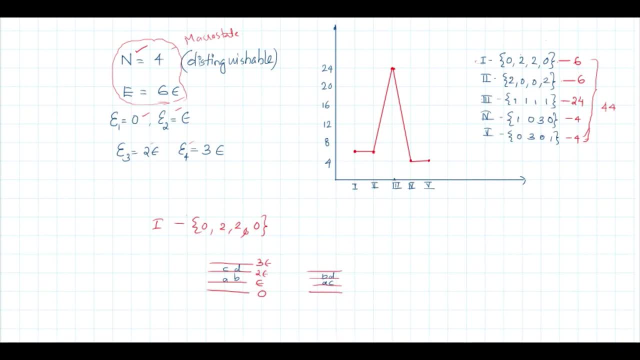 This is the case with four particles. If you increase the particle to say eight, the difference is even greater. For example, if this is eight particles, if we calculate it roughly speaking, the maximum will reach a maximum of 1000,. 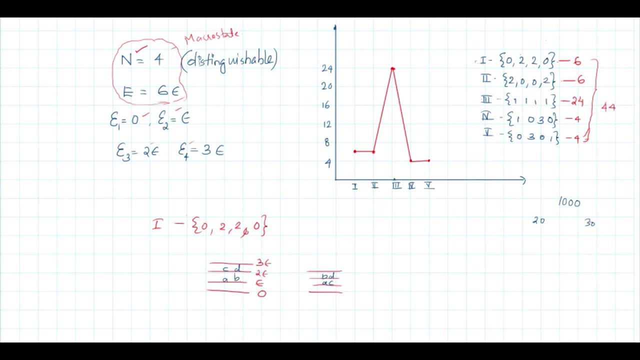 which is in the range of 20-30.. So if a particular distribution is the maximum, then the number of microstates in the most probable distribution will be larger than the rest. The thermodynamic system we consider is the number of microstates in the most probable distribution. 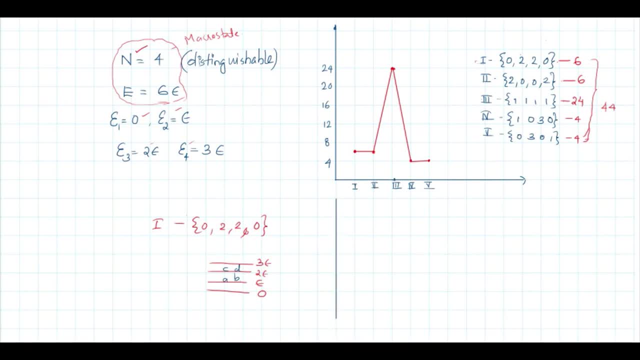 The number of particles and the energy levels in the number of particles will be enormously large. The number of particles: you know, if you take gas molecules in a container, the number of particles will be of the order of 10 to the power 23 per centimeter cube. 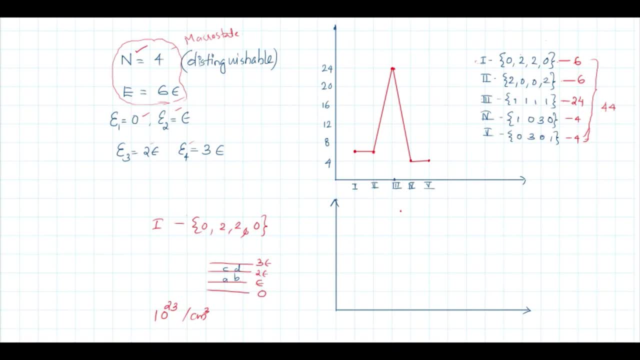 So, when there are so many particles, effectively that graph will be the Dirac delta Around, that Dirac delta peak will be 10 to the power 23.. This is the maximum or most probable distribution. Okay, This graph instead of a width like this: 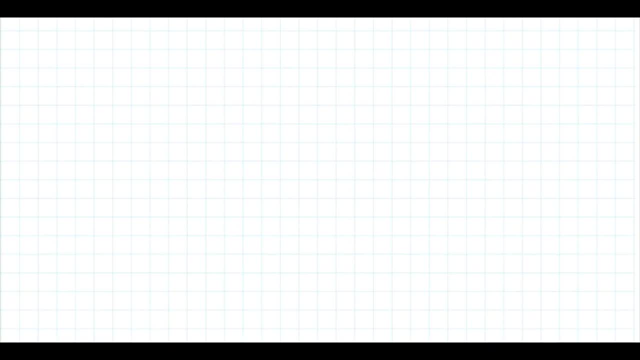 the maximum in a single distribution, the maximum in which the number is infinite when compared to the rest. Otherwise, we will neglect the rest of the distribution. We will neglect the rest of the distribution. So this is the situation Now. as I said in the last lecture: equal a priori probability. 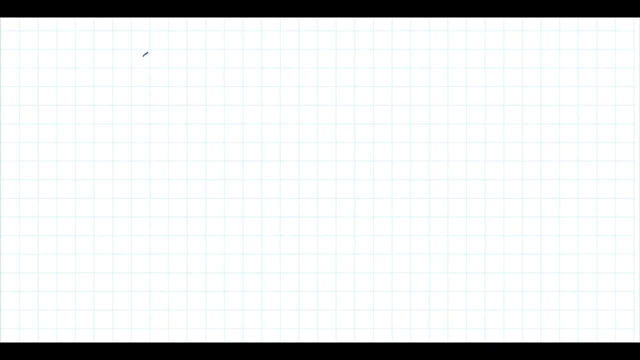 What is equal a priori probability. Equal a priori probability. Equal a priori probability says that all the microstates are equally probable when there is no constraint. If there are no constraints or restrictions in the system, all the microstates are equally probable. 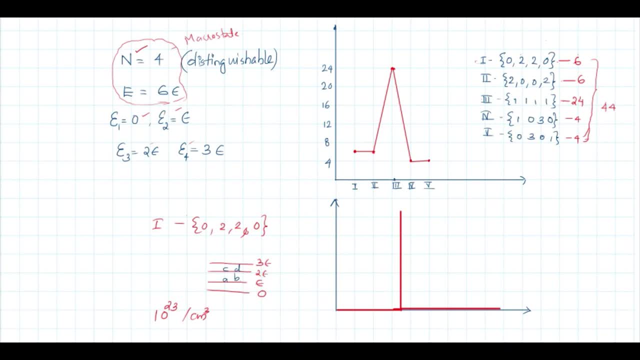 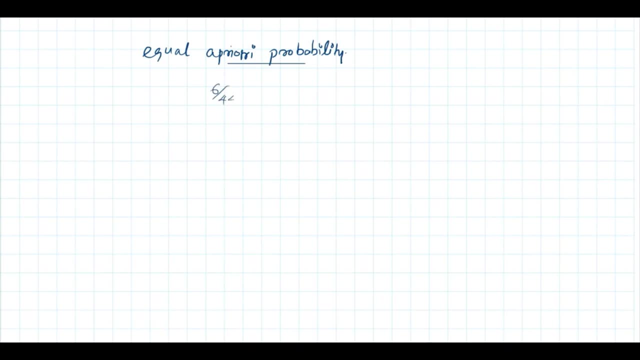 So, if you take the previous example, this is the distribution. The first distribution is 6.. So its probability is 6 by 44.. The total number of microstates is 44. Each one has a probability of 1 by 44.. 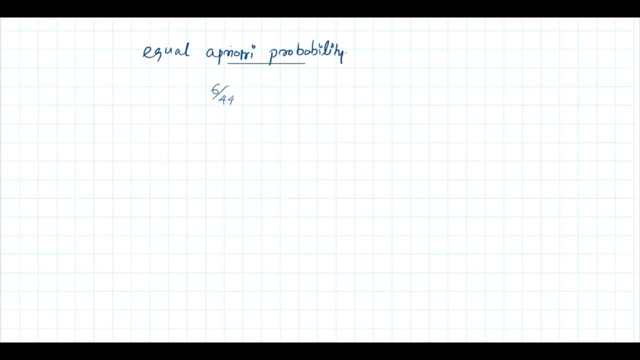 The probability is equal to all. If the total probability is 1, each one should have a probability of 1 by 44. So this distribution has a probability of 6 by 44. The other one has a 6 by 44 probability. 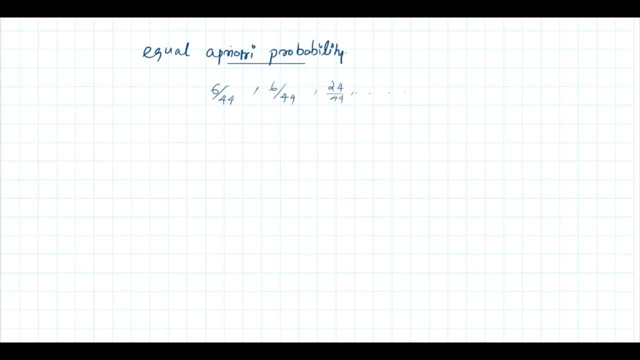 The other one has a probability of 24 by 44. So if, when the number n tends to infinity, this most probable distribution has the maximum number of microstates, So this is the maximum probable one. In this the system has the most probability. 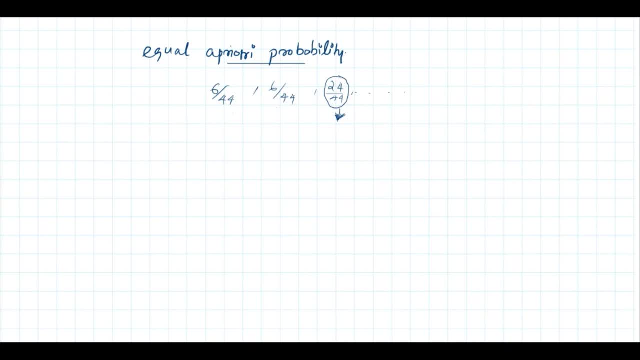 If you have 44 possibilities in this, each one has equal probability. So if you consider it for 1 second, you can think of it as 1 by 44 second, which is divided by 44. The remaining 1 by 44 is in the next state. 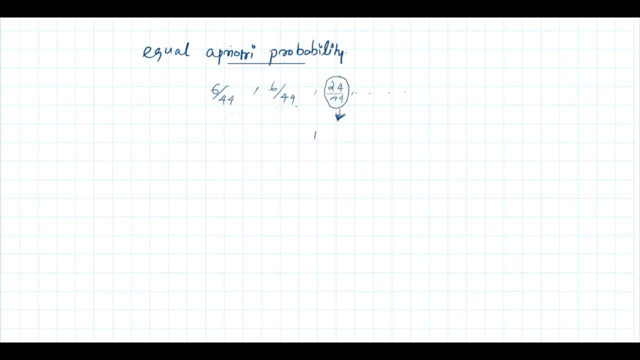 So if it is equally probable in all, if its value is very high, when it tends to infinity, the state where the system spends the most time is the most probable state For that the maximum number of microstates in the system. 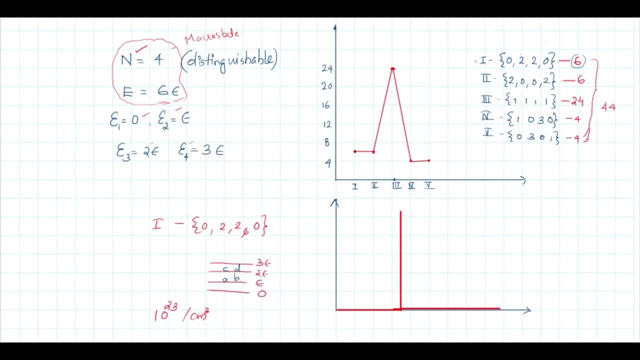 the maximum number of microstates in the system. the maximum number of microstates in the system. this is the distribution For this. since all the other numbers are negligibly small, this is identified as the macrostate of the system. Actually, the macrostate includes all these. 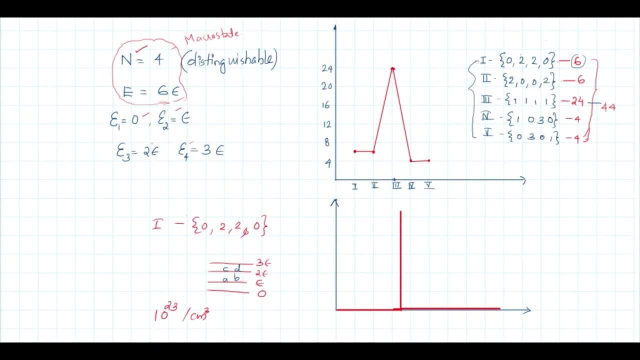 A macrostate contains this much value. There are 44 microstates in it, But according to the increase in your value, the value of the most probable distribution is the most probable distribution, So you can neglect all the rest. The macrostate of the system is: 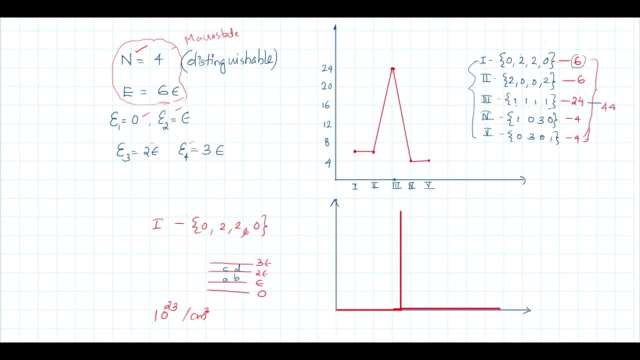 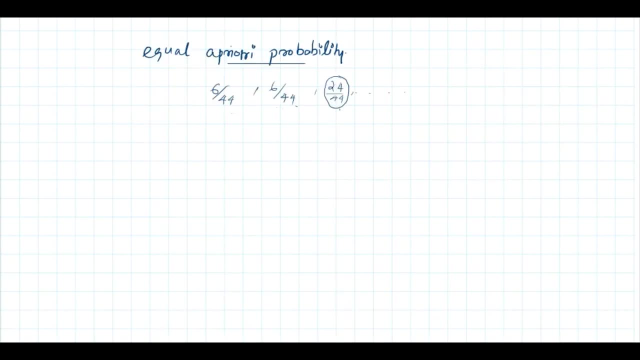 the most probable distribution. The system spends the most time in that state. So that state is called the equilibrium state of the system. So the equilibrium state of a particular thermodynamic system is the one for which the number of microstates is a maximum. 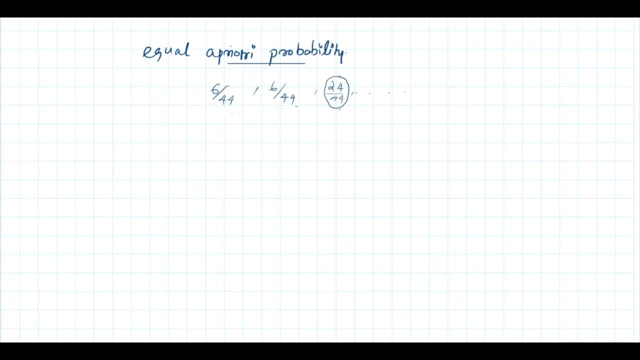 So, if you have a system, if you break the equilibrium state of a system, if you make it not to have equilibrium, when the system goes into equilibrium, the number of microstates will also change. Finally, it will still reach a state of equilibrium. 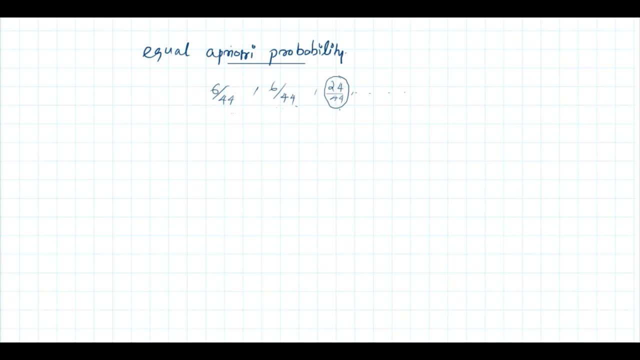 for which the number of microstates is a maximum. So that is the idea. So we can say that for equilibrium, omega 0 should be maximum. That is, omega 0 is a function of E1.. So the first derivative d, omega 0 by d, E1. 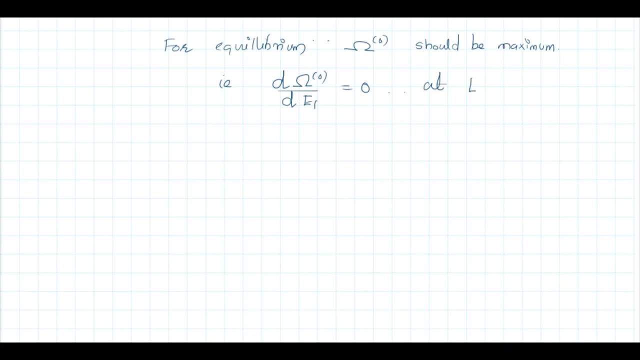 should be 0 at equilibrium. At equilibrium, Let E1 equal to E1 bar be the equilibrium energy. If you represent the energy in equilibrium as E1 bar, I can say that at E1 equal to E1 bar, at E1 equal to E1 bar. 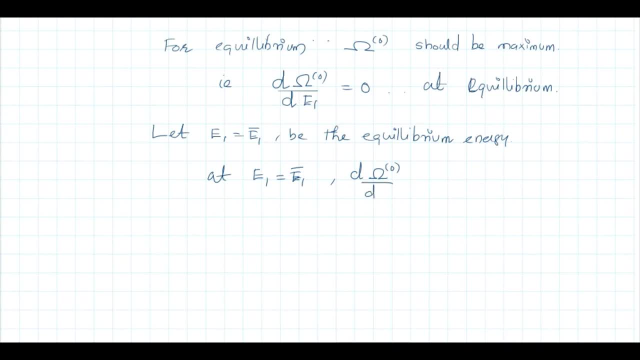 d omega 0 by d E1, d omega 0 by d E1 will be 0.. This is the condition for equilibrium. Now we will derive further d by d E1 of what is omega 0? It is actually omega 1, omega 2,. 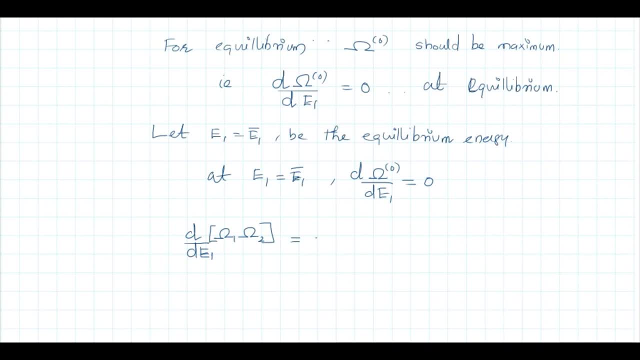 product of microstates of individual systems. Then I can apply product rule d omega 1 by d E1 multiplied with omega 2, plus d omega 2 by d E1 multiplied with omega 1.. But with respect to E1 derivative, 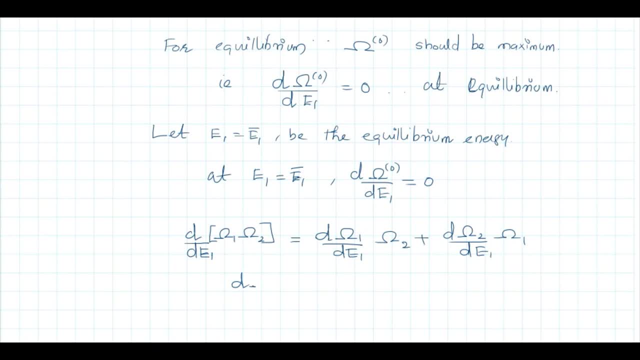 omega 2 is a function of E2.. So I can represent d omega 2 by d E1 like this, using the chain rule d omega 2 by d E2 into d E2, into d E2 by d E1.. 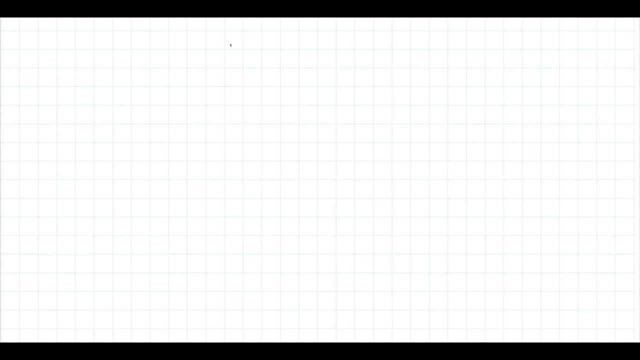 I can write it like this: d E2 by d E1.. But what is d E2 by d E1?? We know that E1 plus E2 is constant. We know that E1 plus E2 is constant. That means d E1 plus d E2 is equal to 0.. 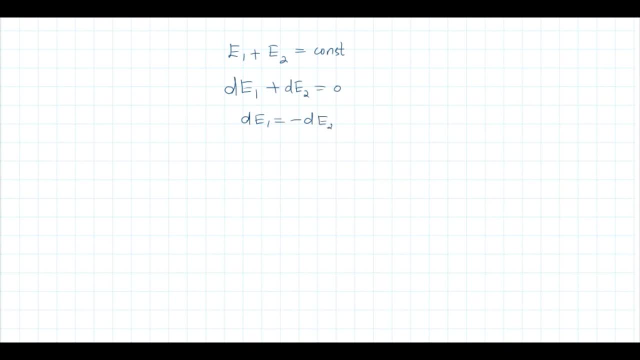 That means d E1 is equal to minus d E2.. That means d E2 by d E1 is minus 1.. Therefore I can write the earlier equation as this should be 0.. This is the equilibrium condition, So I can write it as: 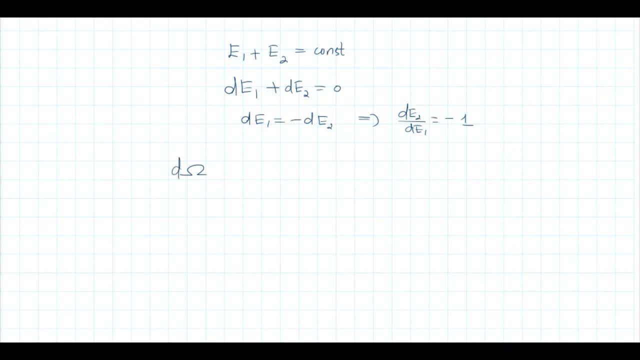 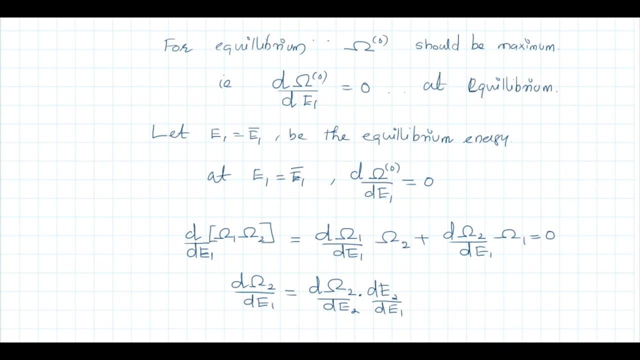 d omega 1 by d E1 into omega 2, minus d omega 2 by d E2 into omega 1, equal to 0.. d omega 2 by d E1, d omega 2 by d E2 into minus 1,. 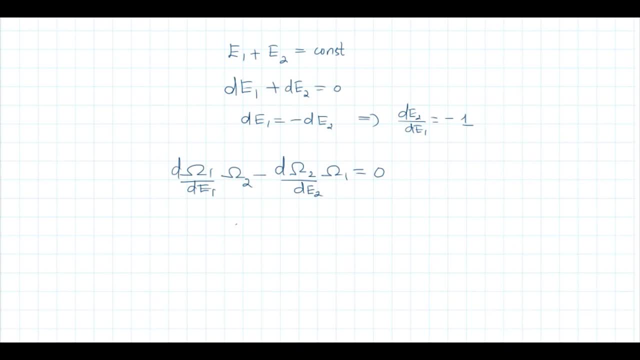 that is why it is minus 1 in the central, equal to 0. This I can write it as: d omega 1 by d E1 into omega 2, equal to d omega 2 by d E2 into omega 1.. 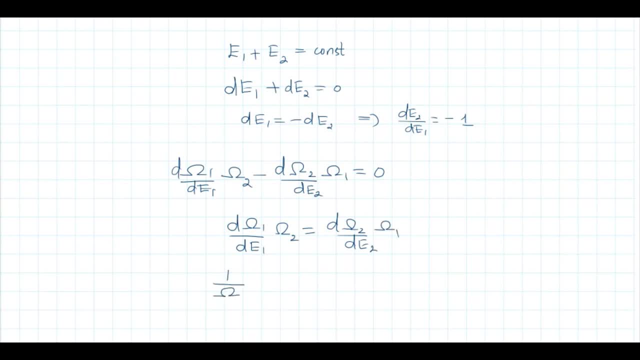 If we exchange the sides of omega 1 and omega 2, it is 1 by omega 1, d omega 1 by d E1, equal to 1 by omega 2, d omega 2 by d E2.. This I can write it as: 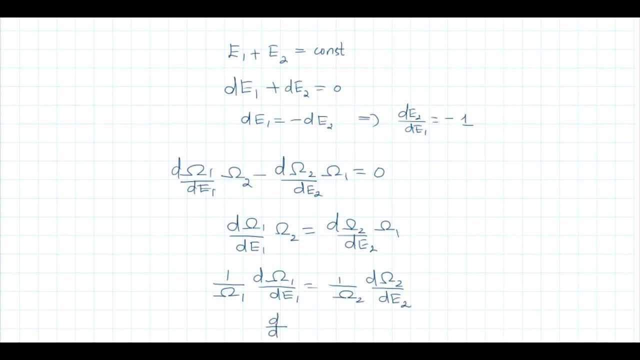 d by d log omega 1 by d E1, equal to d by d E2 of log omega 2.. What is the reason? What is d by d x of log 2 x or the log f? f is a function of x and y. 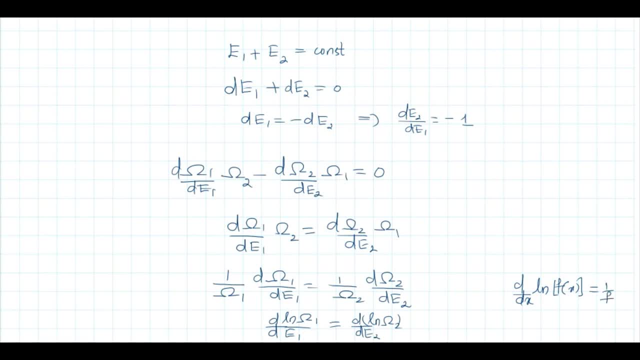 d by d x of log f of x. It is nothing but 1 by f into d x by d x, 1 by f into d x in the derivative, So 1 by f. So here log omega 1,. 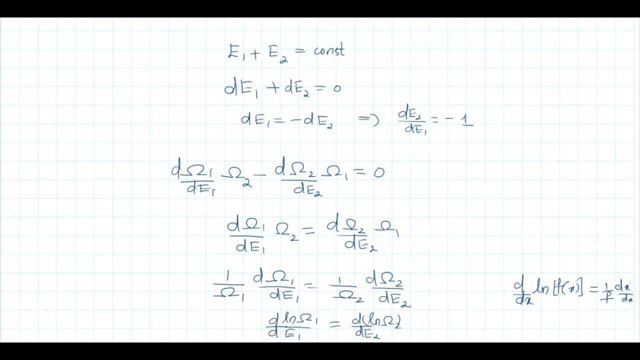 and omega 1 is a function of E1, omega 1 is a function of. oh, this is wrong. actually this is d, f by d x, Log f of x in the derivative. 1 by f into f in the derivative. 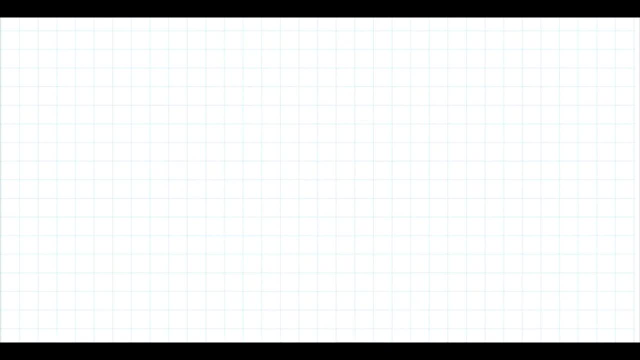 to the respective set d f by d x. So in a similar manner I can write d by d E1 of log omega 1 as 1 by omega 1 into d omega 1, writing here. So left hand side. 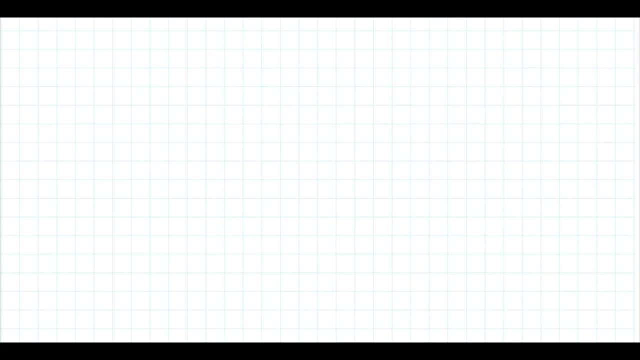 it is for a state system, 1. Right hand side it is for the system 2.. These two are equal means. I can write log omega by log E is a constant at equal Equilibrium, That is dou by dou e of log omega At equilibrium. we are not changing n and v. 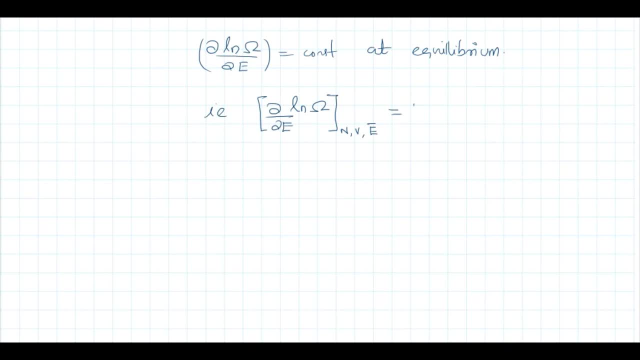 The value of energy is e bar. This is a constant. Let me call that constant as beta. Let this equation be equation 1.. This is equation 1.. This constant is beta over. So that is equation 1.. Equilibrium condition is beta 1 equal to beta 2.. 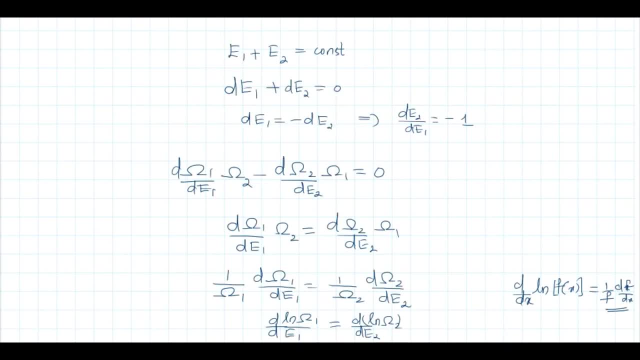 Equilibrium condition is beta 1 equal to beta 2.. Beta 1 equal to beta 2 is the condition of this equation. Here we have written beta 1.. We can call this beta 1.. This is beta 2 of the second system. 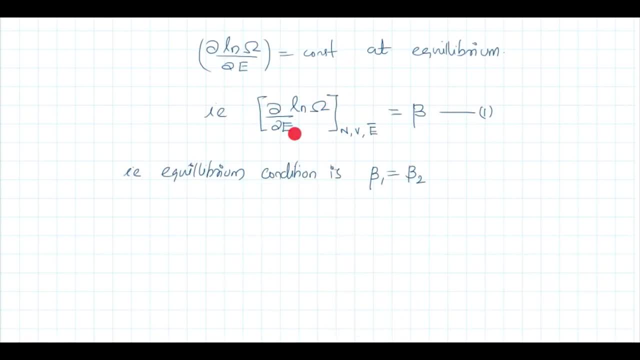 If beta is the value, in the first system, it is omega 1 and here it is e 1.. In the second system, it is omega 2 and here it is e 2. So condition for equilibrium, When you made a thermal contact between two systems, it is beta, 1 is equal to beta 1 is equal to beta 2.. 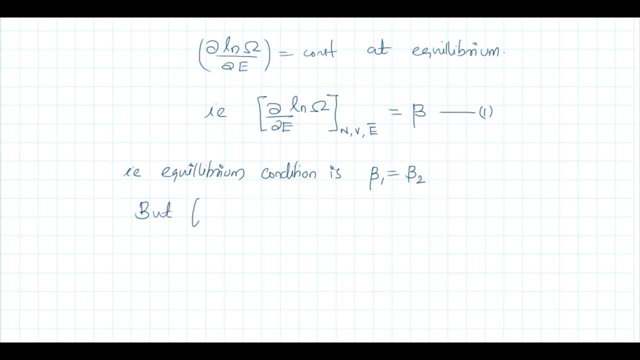 But from thermodynamics we have a relation, We are looking for a connection between statistics and thermodynamics. So we already have an equation. in thermodynamics dE is equal to what is dE in thermodynamics. dE is TdS minus PdV, plus mu dN. 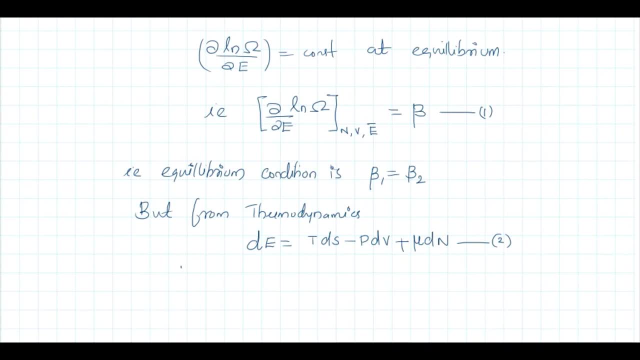 This is equation number 2.. dE is equal to TdS minus PdV, plus mu dN, where T is temperature, T is pressure, mu is chemical potential, S is entropy, V is volume, N is number of particles. 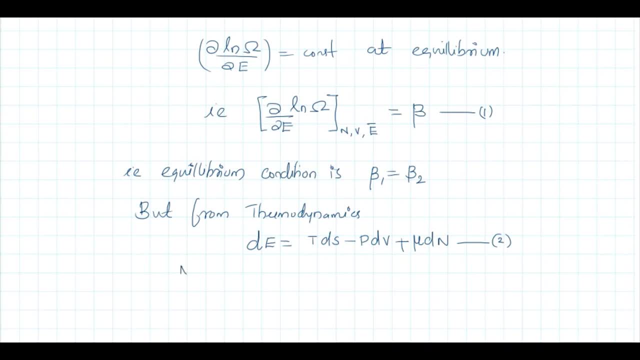 T is the energy of the system. Now N and V are fixed. That is not changed. Implies dE is equal to TdS. So this implies dou S by dou E, dou S by dou E, keeping N and V fixed. N and V fixed is equal to 1 by T. 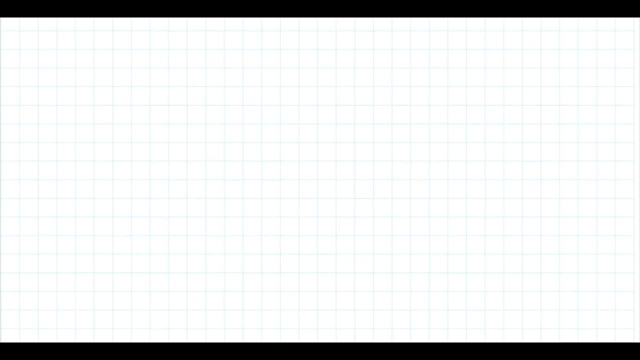 Is equal to 1 by T, Equation number 3.. You can compare equation 1 and 3.. You can compare equation 1 and 3.. There is an intimate relation between the thermodynamics. There is an intimate relation between the thermodynamic quantity, entropy S, and the statistical quantity number of microstates, omega. 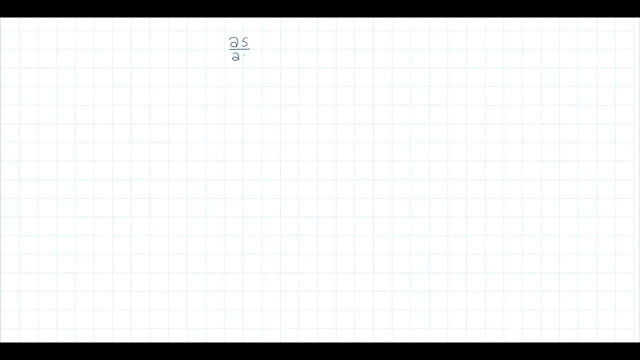 From the two equations. one is dou S by dou E at N V is equal to 1 by T. The other one is dou log omega divided by dou E, again at N V, is equal to theta. So there is an intimate relation between this S and omega. 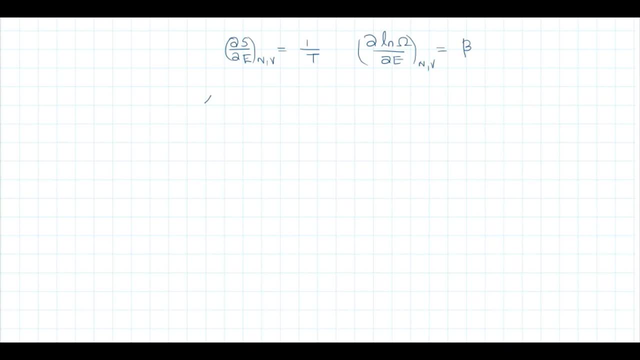 We can write this as some delta S divided by delta log omega. From these two. I can write it as: delta S by delta log omega is equal to 1 by theta Divide these two. okay, And this is a constant. This is a constant for any physical system. 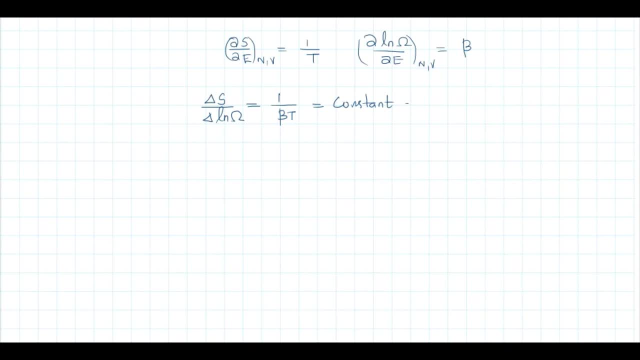 This correspondence was first established by Boltzmann. Okay, So he believed that since the relationship between Thermodynamic approach and the statistical approach seems to be a fundamental in character, This constant should be also a fundamental constant, and that is nothing but Boltzmann. constant K. 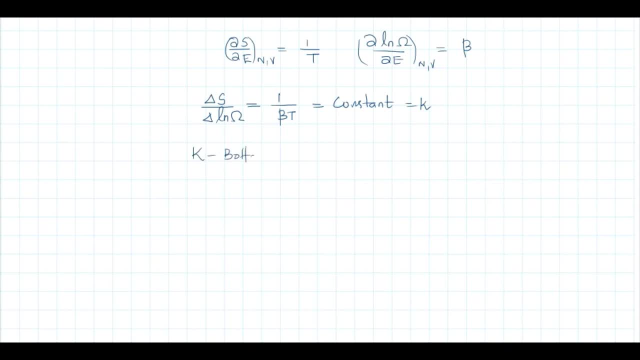 The K is Boltzmann constant. It is a universal constant and its value is 1.38 into 10 to the power minus 23 joules per Kelvin. Okay, Planck wrote the explicit formula: S is equal to K log omega. 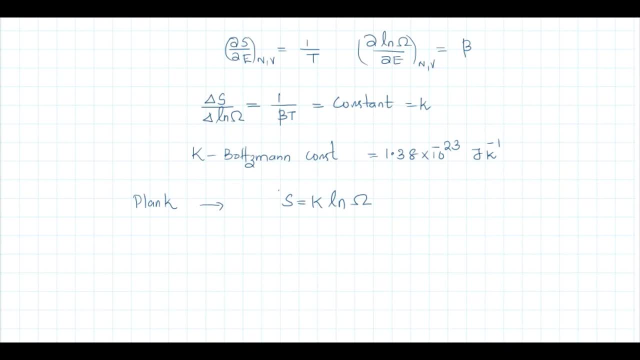 Actually, if you integrate this equation, there will be some additive constant. There will be some integration constant, But Max Planck says that the additive constant will be zero. He explicitly wrote: the relation S is equal to K log omega, Where S is the entropy of the system. 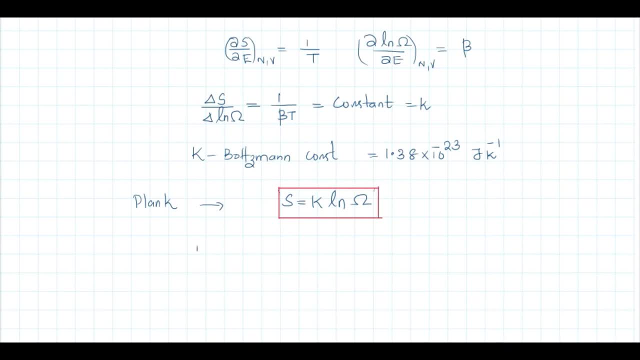 And omega is the number of microstates of the system. So this is the relation between statistics and thermodynamics. S is a thermodynamic quantity, Omega is a statistical quantity: The number of microstates. Okay Now, if omega is equal to 1, that means the absolute value of entropy. S is equal to 0. 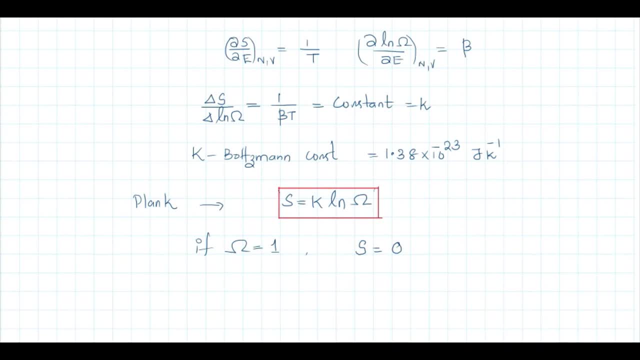 K log 1 is 0. So if omega is equal to 1, that means S is equal to 0.. Omega is equal to 1 means only one microstate for the particular microstate, That is, that microstate is a unique configuration. 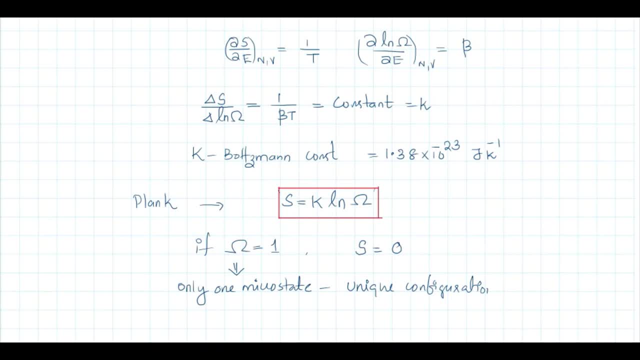 That is a unique configuration. No other choice is existing for the particular microstate, The system in it, the particles in it. That is the only choice. There is no other choice. If there is only one choice, the system can only be in that state. 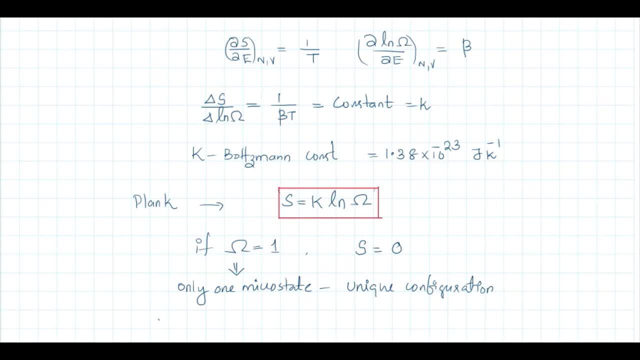 So that is a highly ordered system. That means entropy is a highly ordered system. We do not expect more order in it. There is only one state. The system is always in that state. As omega increases, that means the possible choices for system particles will increase. 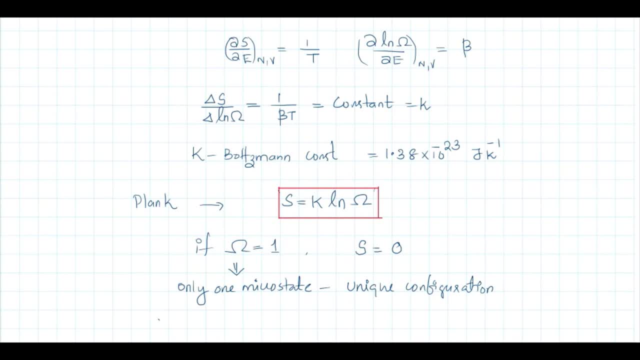 System particles. If you come to a room, if there is only one chair, the only option you have is to sit in that chair. At the same time, if there are 100 chairs in that room, you can sit in one chair if you want. 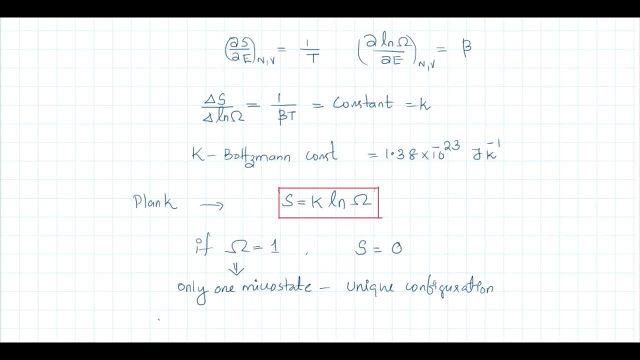 You can go to another chair after a while, So the possibility is higher. That means disorder will also be higher. You can connect the number of microstates as a measure of the disorder in that system As omega increases. as omega increases, S increases. 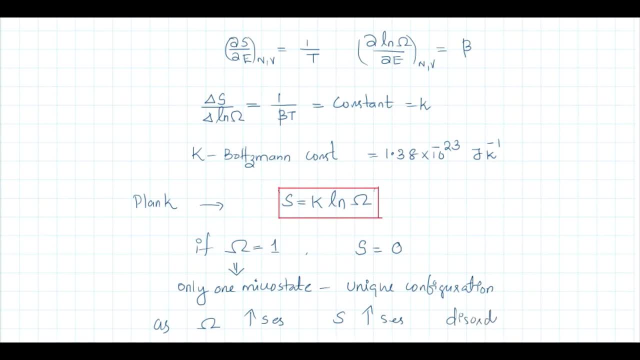 And disorder of the system. How many possibilities exist in that system? according to that, the system is in disorder. If there exists only one unique configuration, the system will always stay in that configuration, And that is a highly ordered state, Whenever the value of omega increases. that is a measure of disorder of the system. 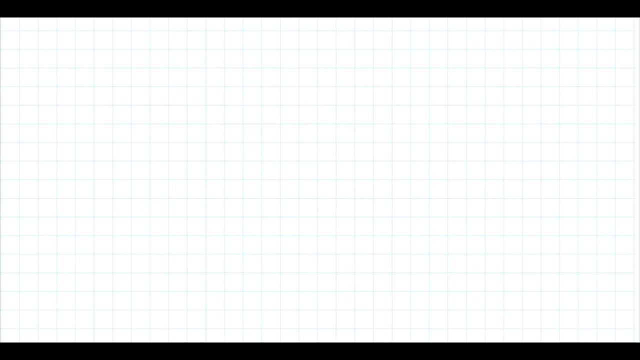 So I can write this beta as beta. Beta is equal to 1 by kT, Because here k is equal to 1 by beta T, So beta I can write it as 1 by kT. Now we will establish further relations between thermodynamics and statistics. 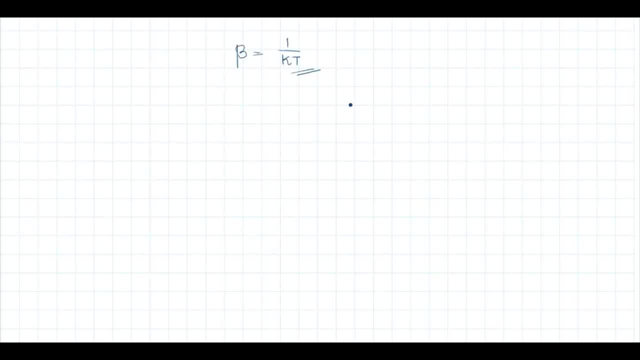 For that we consider the system, the two systems. We already considered two systems And we made the wall conducting in the last. Now we will make the wall also movable. This wall is now movable, also Conducting, as well as movable walls. 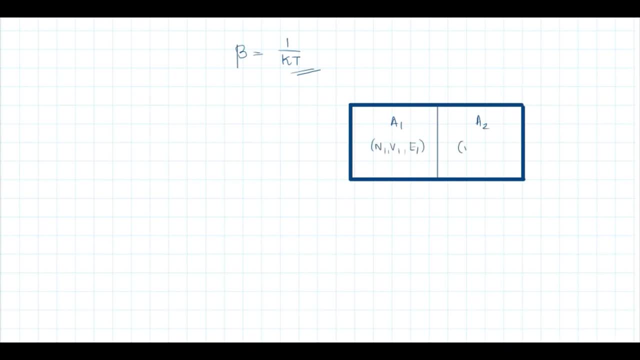 Then what happens is now: there can be change in energy. There can be a change in volume also. When the wall is movable, energy transfer can happen Also. the volume of the system changes, But the total volume Is constant. Now there are two parameters which are constant. 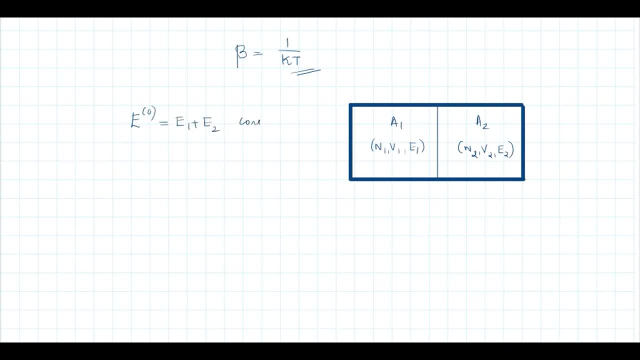 Total energy of the system is constant And total volume of the system. Total volume is V1 plus V2.. It is constant For this combined system. I will denote this combined system as A0.. A0. For that the volume. total volume is constant. total energy is constant. 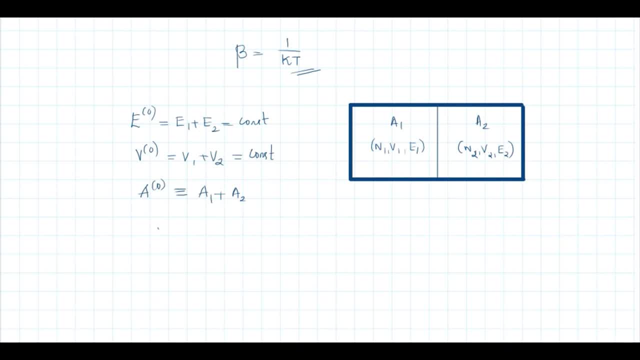 Using the concept of total energy constant, we already Brought an relation dou of log omega 1 divided by dou E1.. At the constant N, N1, V1 and E1 equal to E1, bar Equilibrium value of energy. 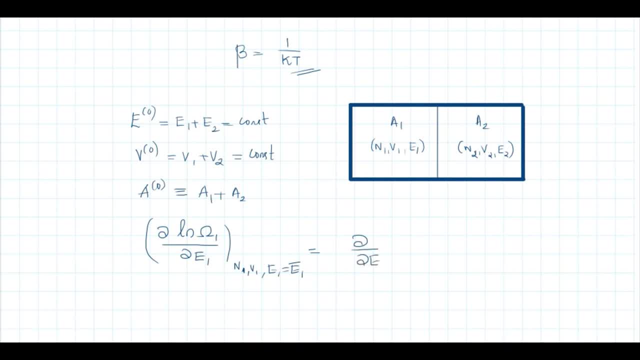 This equal to dou by dou E2 of log omega 2.. And that is for values N2, V2 and E2.. N2 is equal to E2 bar. This relation we established in the last session. Now we will get a similar relation. 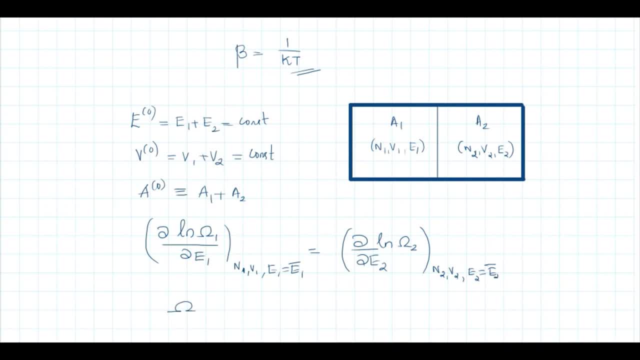 If we take omega as a function of Omega, as a function of V1 and V2.. V2, I can write it as V0 minus V1. So this omega of combined system Will be a function of Omega, of this combined system will be a function of V1 alone. 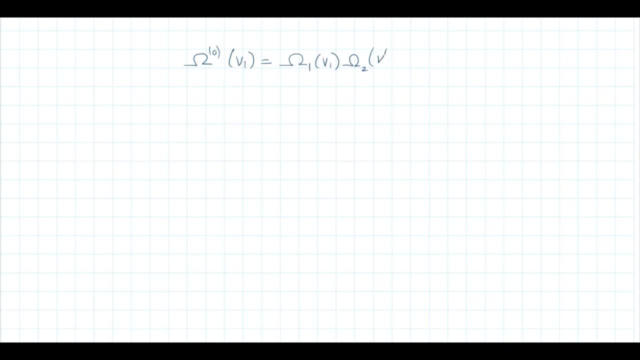 V1 alone. Omega 2 can be written as V0 minus V1.. For the equilibrium: For the equilibrium, we already mentioned that Number of microstates should be maximum. For the equilibrium, I can say that Dou, omega of 0 divided by dou V1 is equal to 0.. 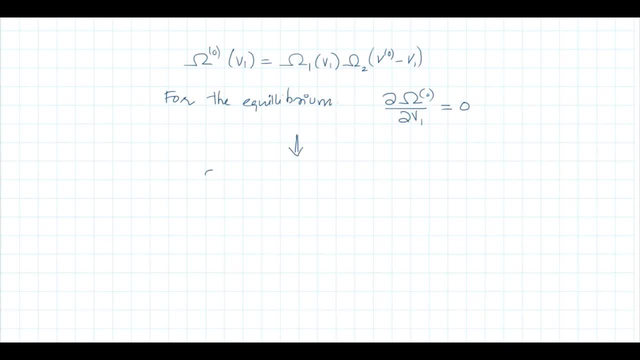 This will yield me a relation like dou of log omega 1 divided by dou V1 at N1, E1 and V1 is equal to V1 bar Equilibrium volume, And dou by dou V2 of log omega 2 at N1. 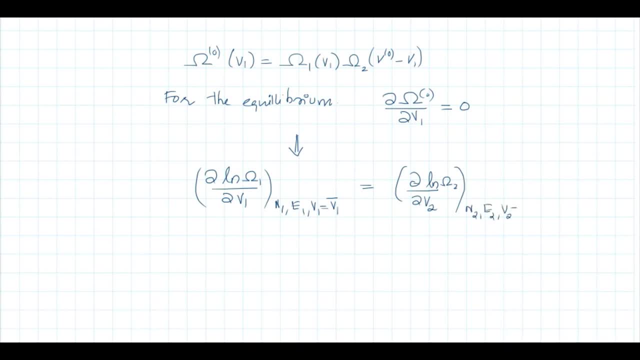 N2, E2, V2 is equal to V2 bar. Okay, So, using this concept, Changing volume will change the number of microstates And it will continue up to the equilibrium state, And the equilibrium state is the one for which the number of microstates is a maximum. 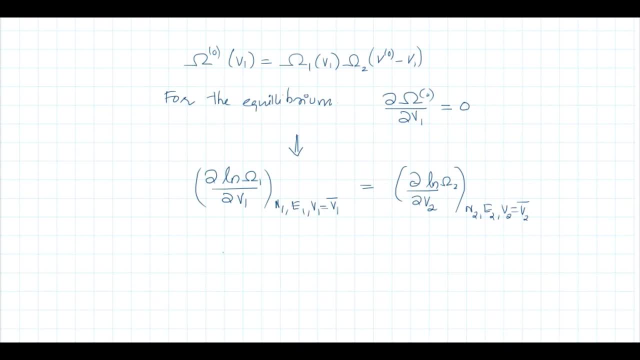 So, using thus that relation, we can establish an equality of these two And I can call this constant as constant value, As eta That is. I can write: Eta is equal to dou by dou V of log omega at constant N, E and V equal to V bar. 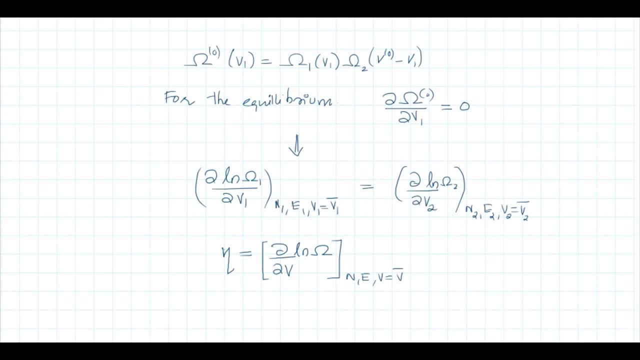 Okay, This quantity, eta, we obtained using the concept The equilibrium will achieve by changing the volume, And equilibrium means the volume At which the number of microstates is maximum. We already have from the energy, from the values of variation of energy. we already have dou by dou E of log omega at constant N, V and E equal to E bar as beta. 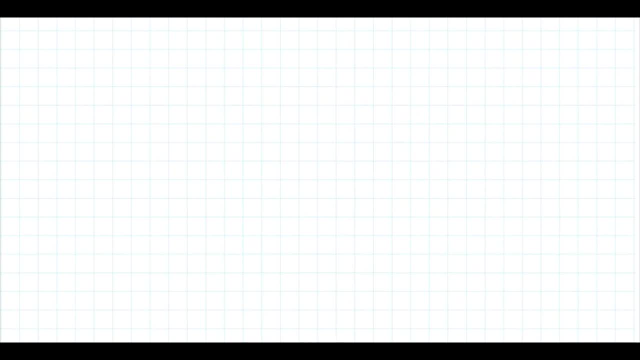 So we now have two values, eta and beta, For equilibrium of the system, For equilibrium of the combined system. We had two systems. Those two systems were in separate equilibrium. After that their interlocking wall was made conducting and movable. Conducting and movable. 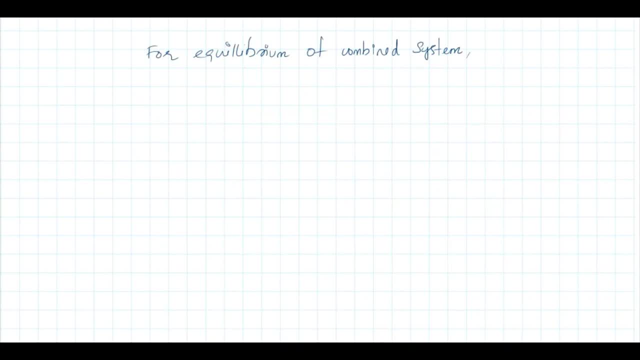 At that time when will we reach a new equilibrium state? For equilibrium of combined system We have: beta 1 is equal to beta 2 and eta 1 is equal to eta 2.. Now suppose the wall is permeable to particles also, that is, energy can exchange between the two systems. volume can vary between the two systems. it is movable. 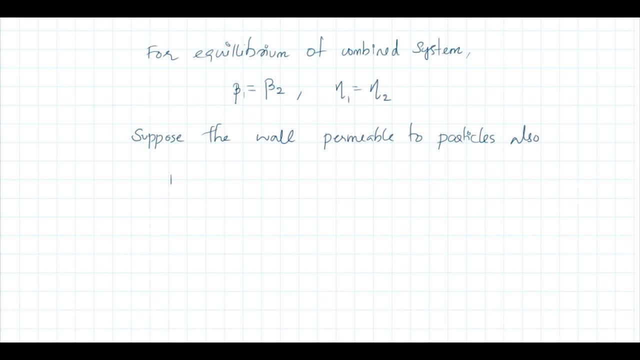 Now it is permeable to the particles also. Now it is permeable to the particles also. The particles from first system can move to the second. Our particles from second system can move to the first one. The wall is permeable to particles. 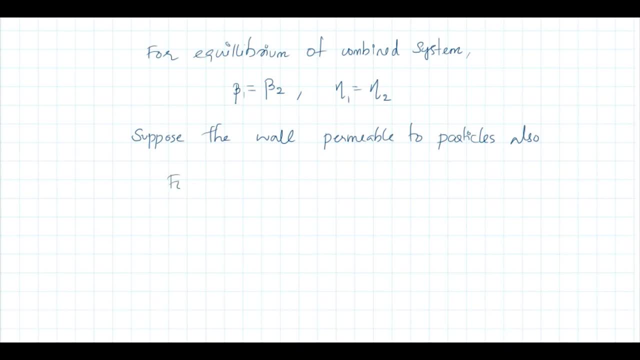 Then for the combined system. for the combined system, I can write omega of 0 as a function of N1, as a function of N1.. It is omega 1, N1 into omega 2.. It is N0. It is N0 minus N1. 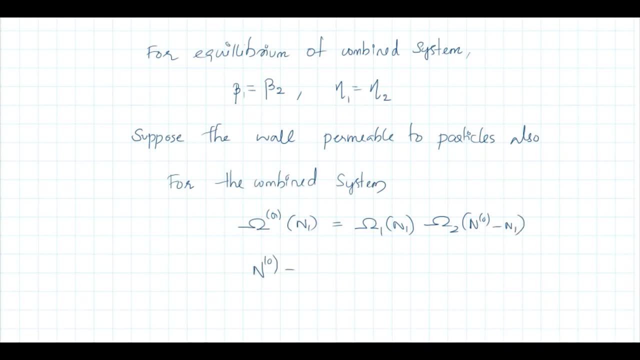 Total number of particles is fixed. N0 is N1 plus N2.. It is fixed, It is constant. So this omega is a function of N1 alone. By varying N1, you can make omega value vary, And equilibrium state is the one for which number of microstates omega 0 is a maximum. 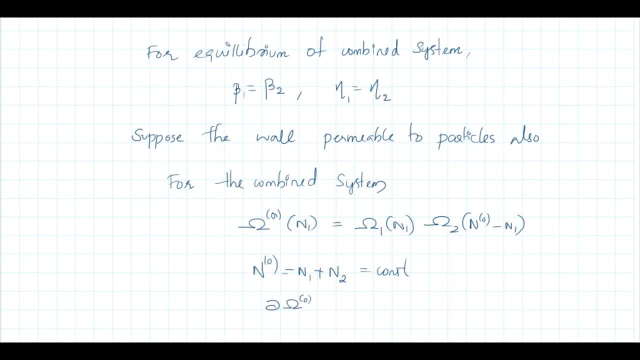 And we can write dou: omega 0 divided by dou N1 is equal to 0 at equilibrium. This condition will give me a relation similar to the previous two cases. We have already written the energy gain and Celsius And this will give me a relation like dou by dou N1 of log omega 1 at V1- E1 and N1 is equal to N1. bar is equal to dou by dou N2 of log omega 2 at V1- E1.. 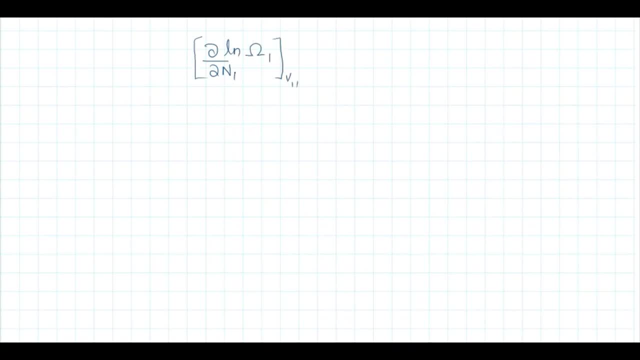 And N1 is equal to N1. bar is equal to dou by dou, N2 of log omega 2 at V2 E2, N2 is equal to N2 bar. So this equality should also be satisfied. for the equilibrium That is, I can introduce a new parameter. 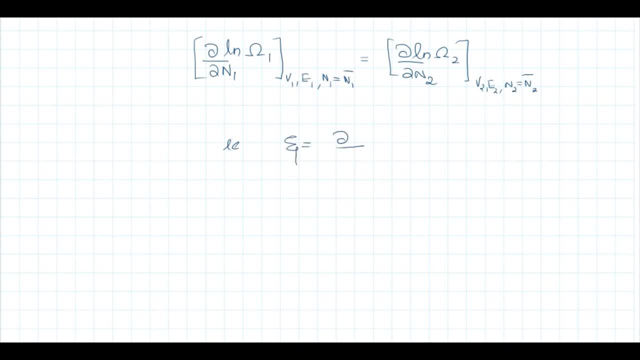 It is theta, which I will denote it as dou by dou: N of log omega at the constant VE and N equal to N bar. This is theta, Then, for complete equilibrium of system. for complete equilibrium of the system, complete equilibrium of system. I will call that equilibrium as thermodynamic equilibrium. 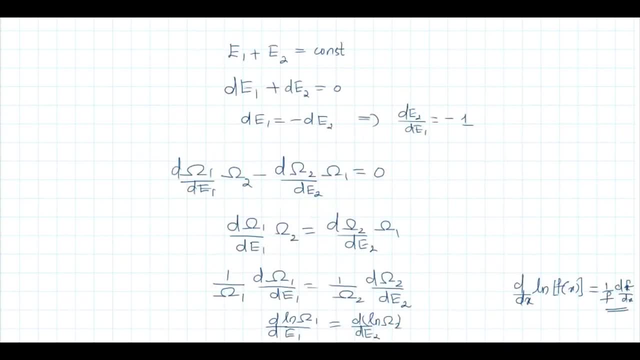 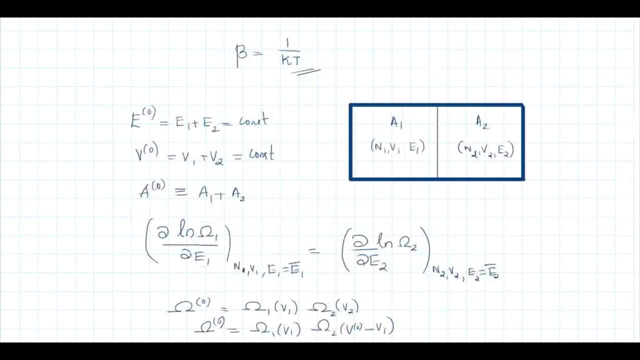 The first one. when you can weigh Only the energy, the equilibrium attained is called the thermodynamic equilibrium. When you can change the volume also, the equilibrium achieved is called the mechanical equilibrium. When you can change the number of particles, the equilibrium achieved is called the chemical equilibrium. 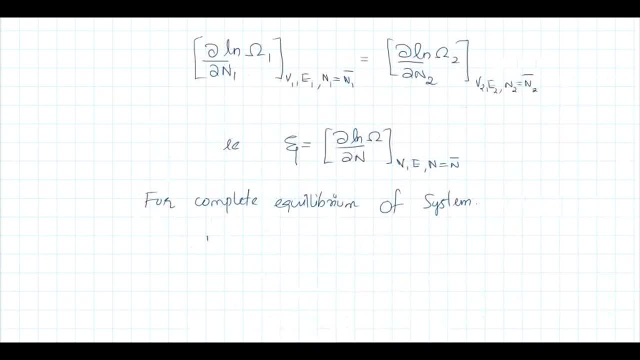 When all the three equilibriums are achieved, the system can be said to be in thermodynamic equilibrium. And for the complete equilibrium we can write: beta 1 is equal to beta 2.. Beta 1 is equal to beta 2.. 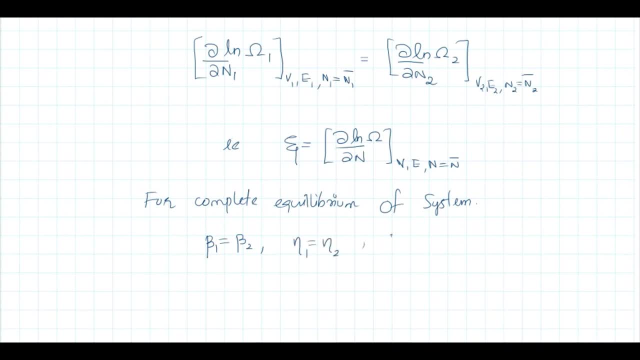 This is the condition for complete equilibrium of the system. Complete equilibrium of the system. We already established that beta 1 equal to beta 2 implies 1 by kT1 is equal to 1 by kT2.. That is T1 equal to T2.. 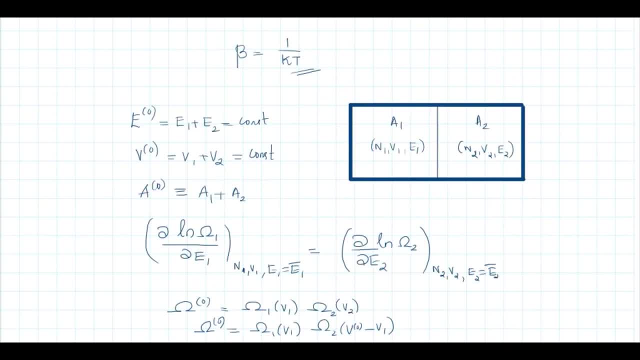 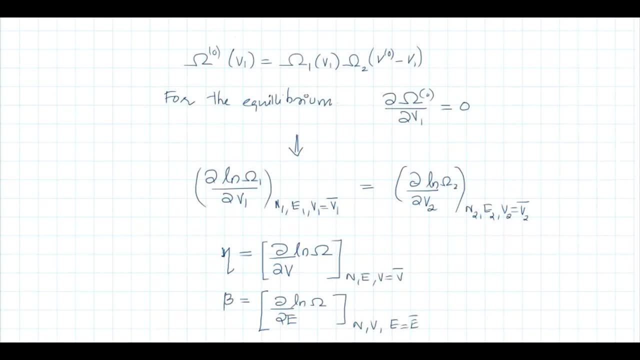 So when you have a, When you have a system which is separated by a conducting wall, there will be transfer of energy between the system until the temperature of the two systems is constant. That is our idea from thermodynamics. Okay, From thermodynamics, we know that if we made a thermal contact between two systems, heat energy will flow from one system to the another until the temperatures are equal. 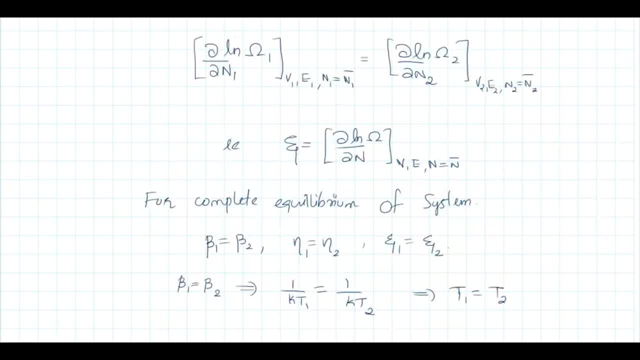 In a microscopic point of view or a statistical point of view, That condition is beta 1 equal to beta 2.. And that is equivalent to saying that T1 equal to T2.. So what is the corresponding equivalency for eta 1 equal to eta 2 and zeta 1 equal to zeta 2?? 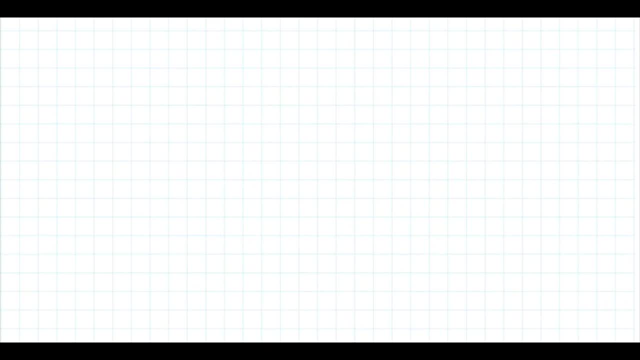 If we say beta 1 equal to beta 2, that means temperature is equal. Can we bring the same kind of correspondence to these parameters? If we can, what will happen? That is what we are looking for Now. let's see. 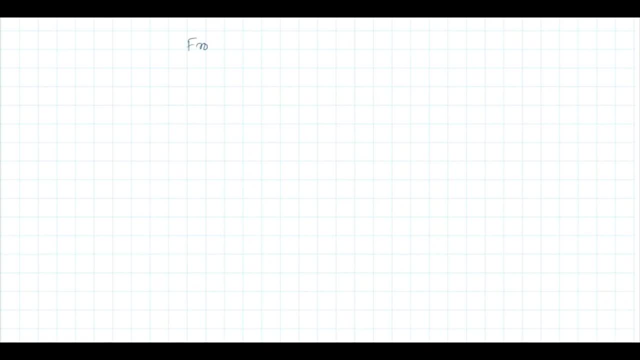 From thermodynamics we can say that temperature is equal to T1 equal to T2.. So what is the corresponding equivalency for eta 1 equal to eta 2 and zeta 1 equal to zeta 2?? We can use the thermodynamics relations to get the temperature. 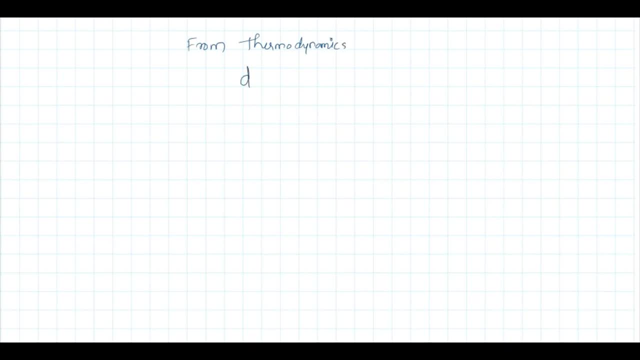 From thermodynamics we already wrote an equation like d is equal to TdS minus PdV plus mu. dN In this eta is obtained when we took the case of the second volume. So for that we keep N and E fixed. 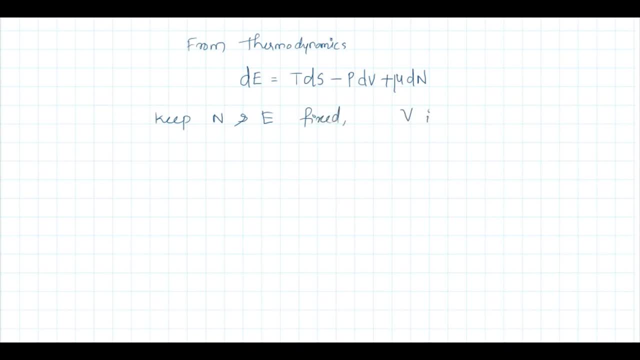 B is varying. B is variable, Only the volume varies. In that case, if we fix N and E, I can write it as TdS minus PdV equal to 0.. Or dou S by dou V at constant NE, as P by T. 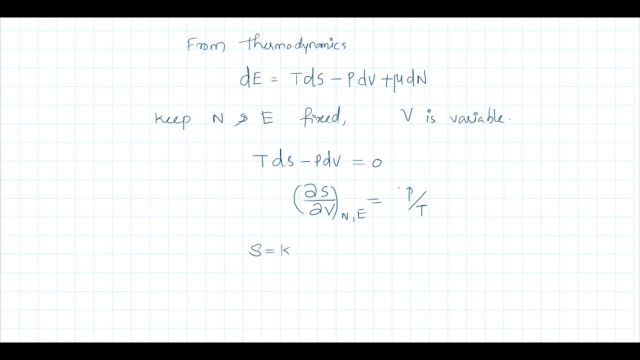 But we already have S equal to K log omega, S equal to K log omega, So I can write it as dou log omega divided by dou V at constant NE, as P by KT. dou log omega by dou V at constant NE. What did we call that? 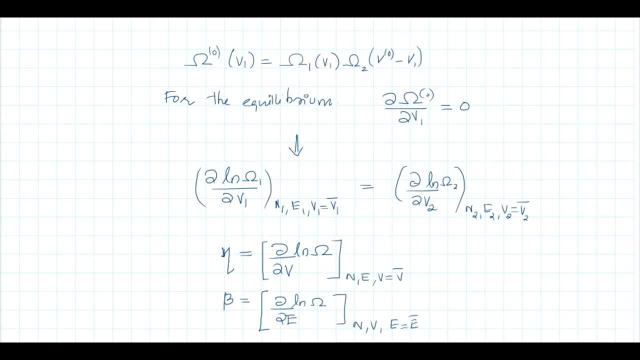 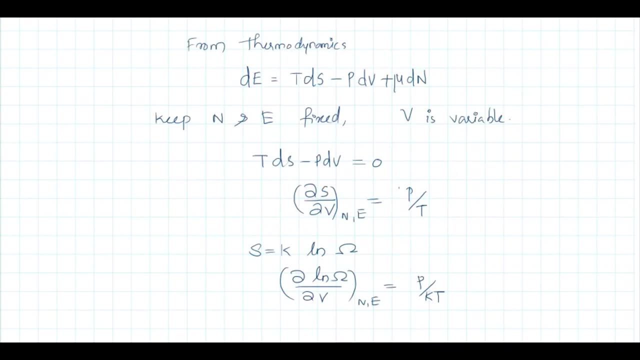 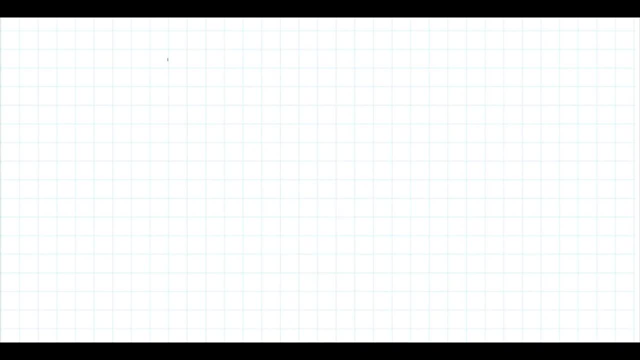 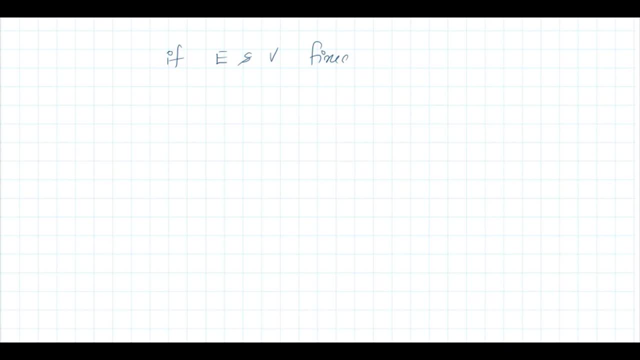 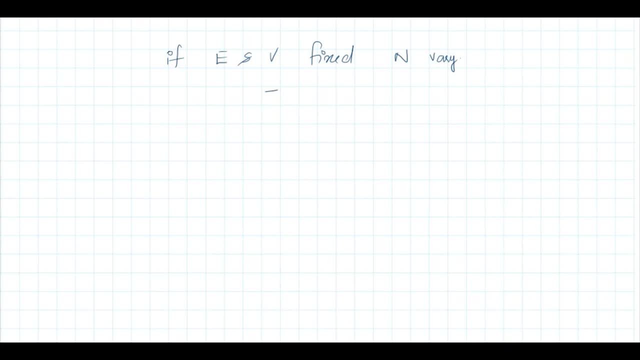 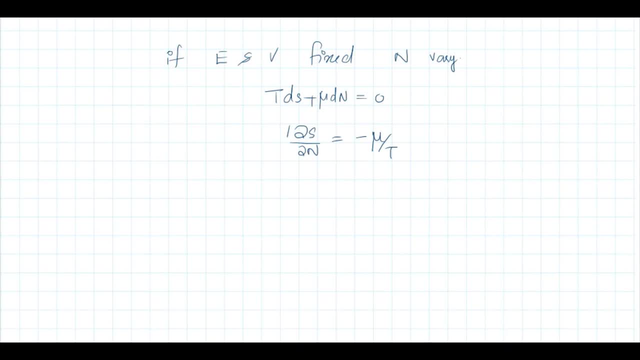 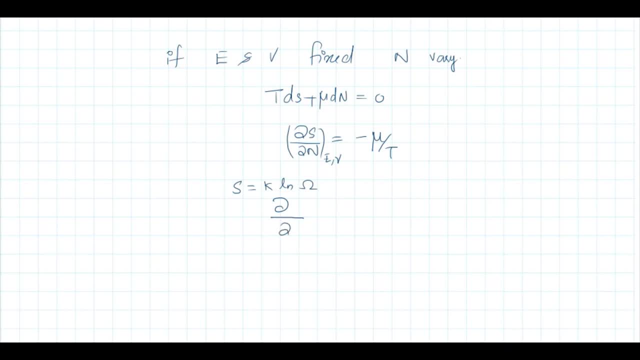 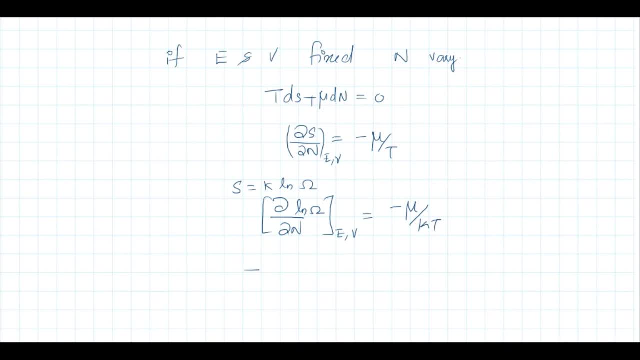 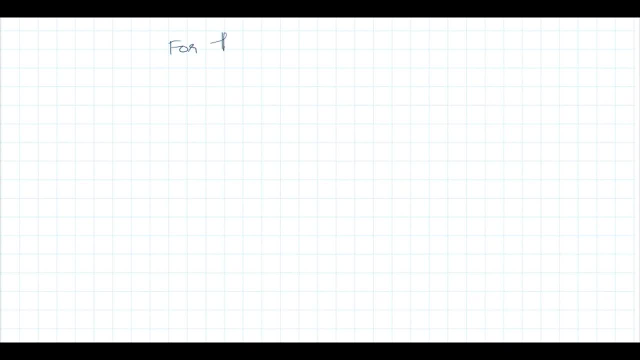 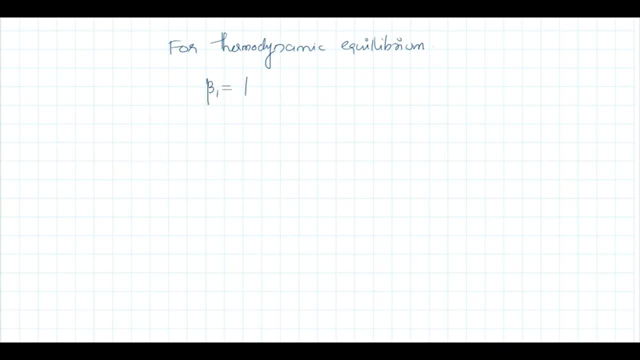 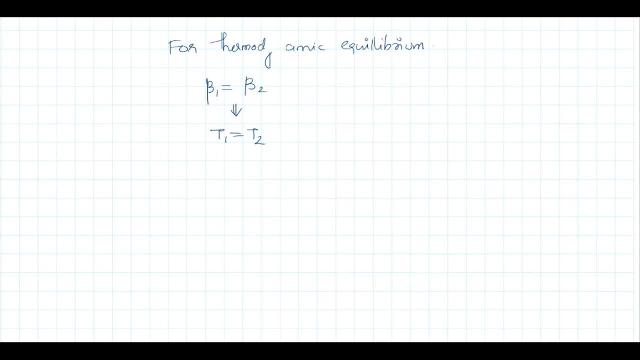 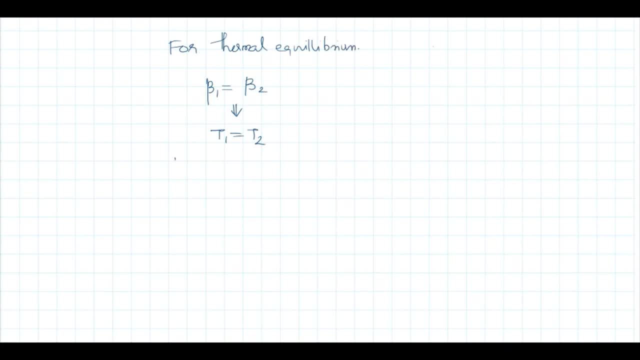 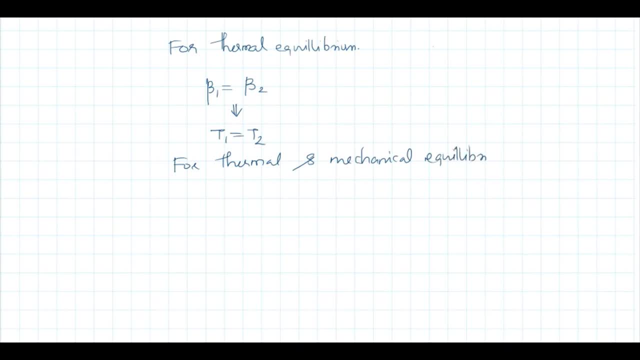 mechanical equilibrium can be achieved. thermal and mechanical equilibrium can be achieved by the equality of two parameters: beta 1 equal to beta 2 and eta 1 is equal to eta 2. that is, t1 is equal to t2. also p1 equal to p2. what is eta? eta is actually p by kt when k and t are constant. 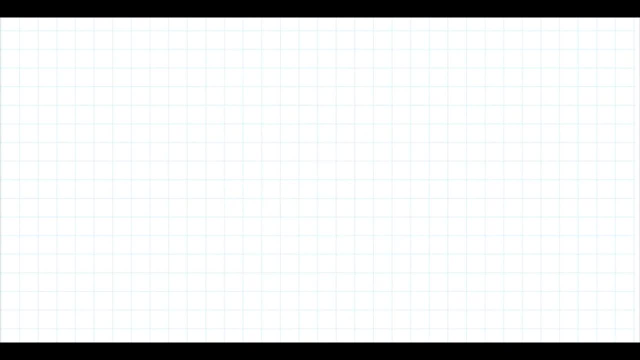 eta 1 equal to eta 2 means p1 equal to p2. so the system will have a mechanical equilibrium and the pressure of both sides are equal, or the wall between the systems will move until the pressure on both sides are equal. then the pressure equal of the number and the wall will move you. 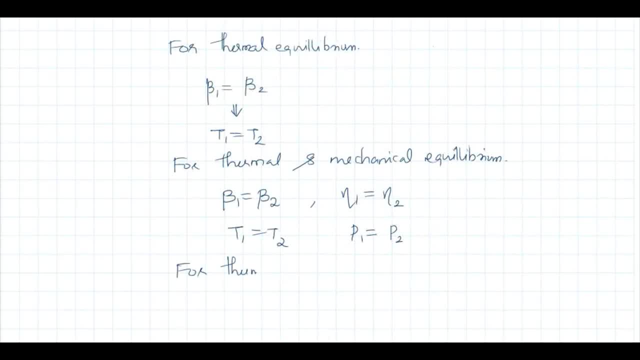 now for thermal, mechanical and chemical equilibrium. chemical equilibrium: number of particles in a infinite time to move, without the particular state that will stop you, and that is called the chemical equilibrium. then you have beta 1 equal to beta 2, eta 1 equal to eta 2. 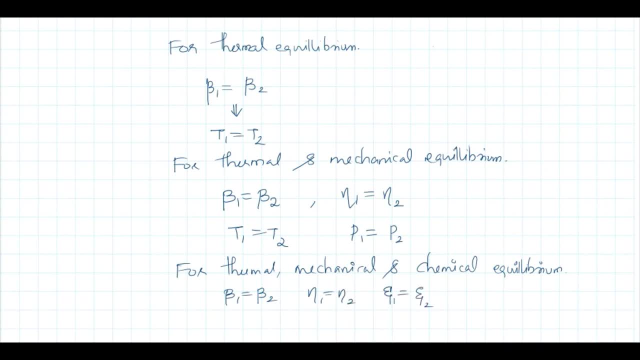 zeta 1 equal to zeta, that is, t1 equal to t2, p1 equal to p2 and mu 1 equal to this is the condition for a complete equilibrium. when you have two systems, okay, they are separately in equilibrium. there. we made a contact between them, okay. 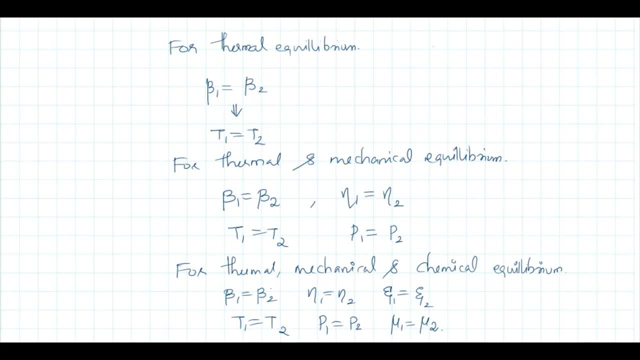 energy can vary, number of particles can vary, volume can be okay when all these three parameters can vary. finally, a state of equilibrium will be achieved when these three are equal: beta, eta, zeta, and that is equivalent in saying that e, p and mu are equal. this is thermodynamic version. 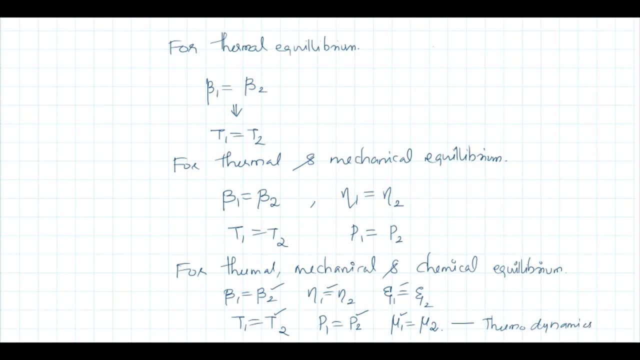 and this is a statistical version. so now we are ready with the tools for deriving thermodynamics from statistical point of view. we have the equation: s is equal to k log omega, where omega is a function of n, v and d. E It is the number of microstates of a particular system. S is the entropic, K is the Boltzmann. 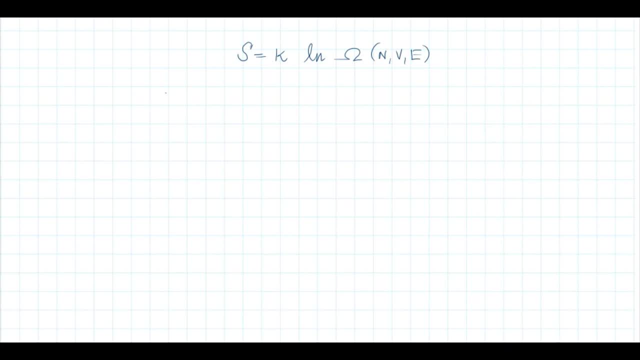 constant. This is the connecting link between statistical parameter omega and the thermodynamics parameter S. We also have these equations: dou S by dou E at a constant n and v is equal to 1 by t, and dou S by dou v at a constant n, e as p by t. dou S by dou n at a constant v e as minus mu by. 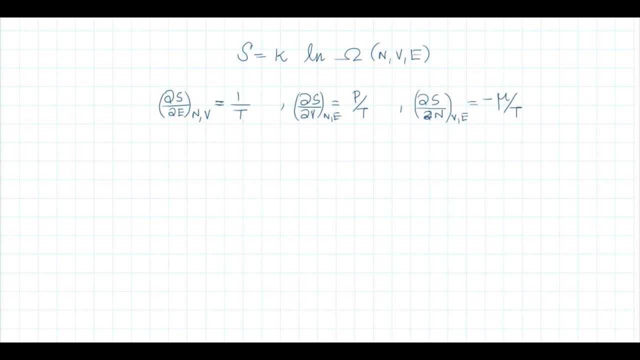 t All these relations we already derived. So once we have the relation S equal to K log omega, with omega already calculated, you can find S entropic as a function of n, v and e. Using that, we can find this intensive parameters: temperature, pressure and chemical potential. 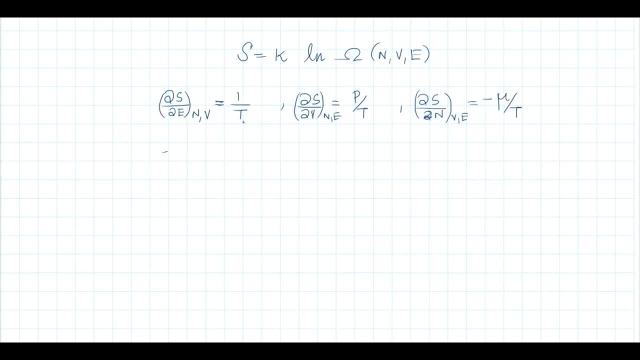 using this relation, By taking partial derivative with respect to E, we can find temperature. inverse of temperature. By taking the partial derivative of S with respect to v, keeping n and v fixed, we can find p by t, finding the partial derivative of S with respect to. 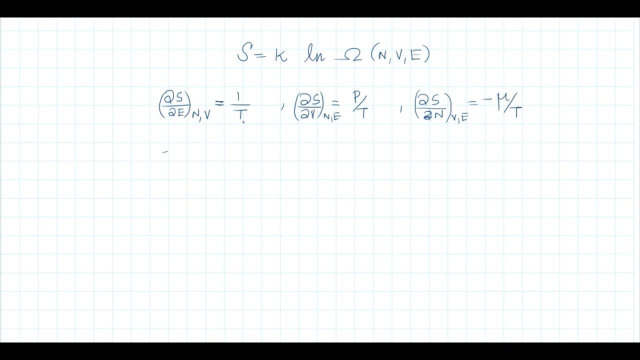 n, keeping volume and energy constant. you can find minus mu by t, So you can find this. intensive parameters, temperature, pressure and chemical potential. You can find this. Sometimes the given quantity may be total energy, energy of the system, and it is given in terms of, say, n, v and s. okay, you can invert this relation. 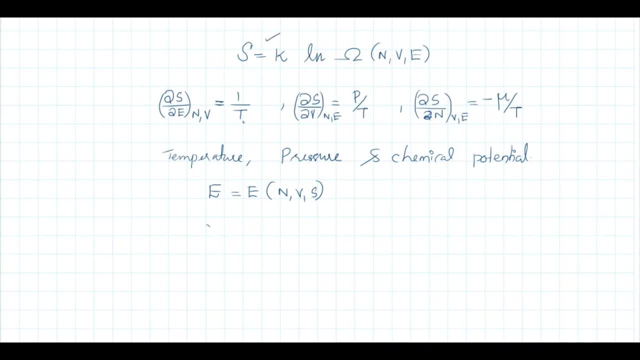 s is a function of n, v and e. you can invert this relation in principle, so you can write e as a function of n, v and s. we already have this relation: t d e equal to t d s minus p d v plus mu d n, t d s minus p d v plus mu d n. so i can write dou e by dou e by dou v. 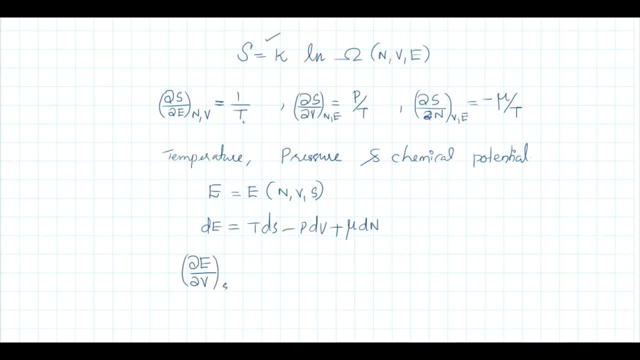 at constant s and n, of course you have. take the partial derivative with respect to v. keeping s and n constant, then this t d s becomes 0, mu d n becomes 0. you can see that it is nothing but minus p. also dou e: by dou s keeping v and n constant, this d v is 0, d n is 0. dou e by dou s will give you. 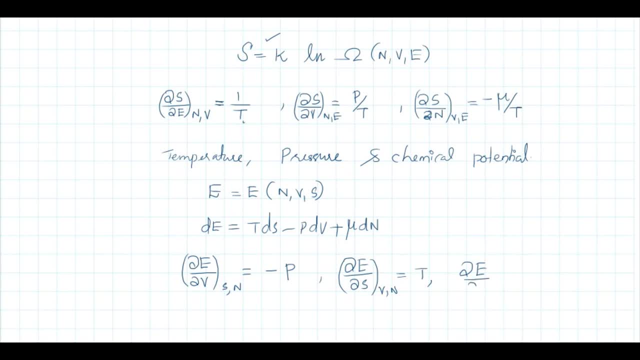 t. also dou e by dou n at the constant s v. that will give you at constant s v mean d s is 0, d v is 0. so dou e by dou n will give you the value of mu. okay, so you can use this relation also. 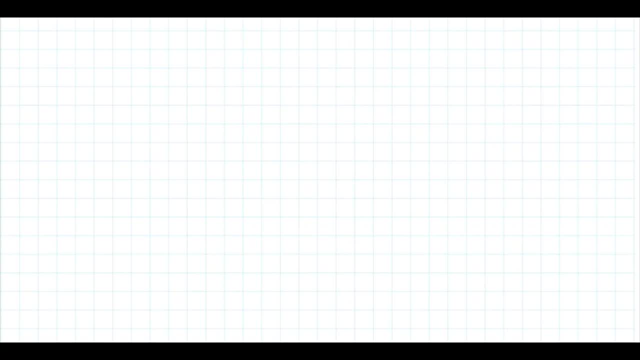 okay for finding this: pressure, temperature and chemical potential. for finding the rest of the thermodynamics this straightforward, i will give you a easy way to memorize the equations. let the variables- thermodynamic variables- be pressure p, volume v, temperature t and entropy. s okay, and the thermodynamic functions: thermodynamic functions. 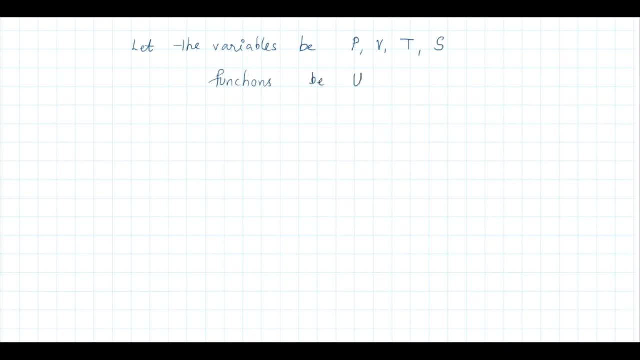 the internal energy u. okay, instead of e i will use the letter u, then helmholtz free energy f, then enthalpy h, and it gives free energy g, because these are the thermodynamic functions, these are the thermodynamic variables. then 같이告诉你我们可以用这个ador. 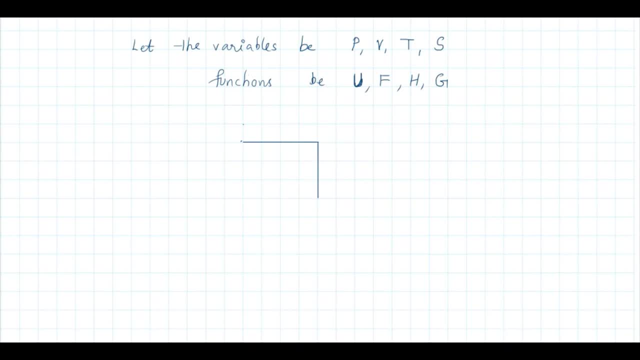 你可以用这个ador 可以用这个: utilized this diagram 是这样大的代表: Thumb 这个 然后在这里 在这里 Ich record. 你可以在这里. Here you can write B. Here you can write H. Here you can write S. 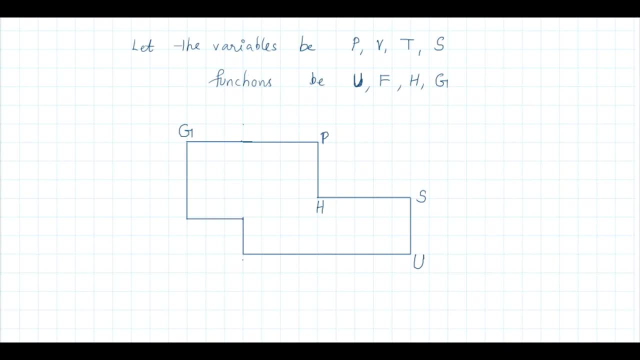 Here you can write U. Here you can write V. On this corner you can write F. Here you can write T. Now, how can you Memorize these things? G, you can write it, as good. physicists have studied under very fine teachers, so, using this script, you can memorize these. 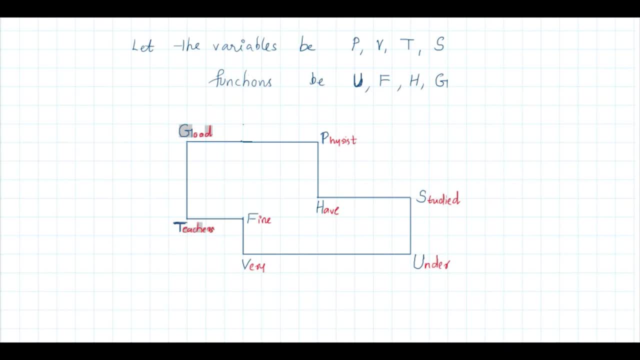 quantities. but remember to start from this, this point, okay, otherwise this will then draw. so this is this: g is Gibbs free energy, p is pressure, h is enthalpy, s is entropy, u is internal energy, v is volume, f is Helmholtz free energy, t is temperature. 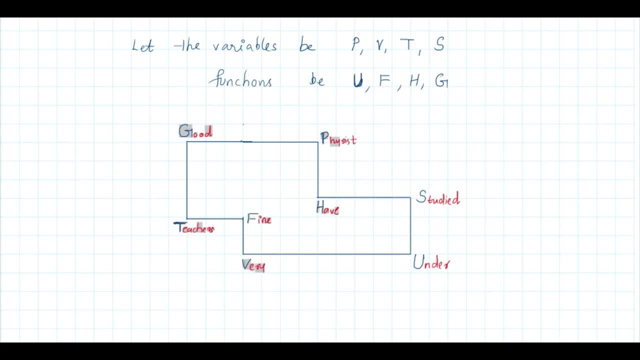 now, what is the significance of this diagram? what is the significance of this diagram? look at these functions. I can write, for example, this: u internal energy u. it is a function of. it is a function of the variables which are nearer to it. okay, the u in the left. 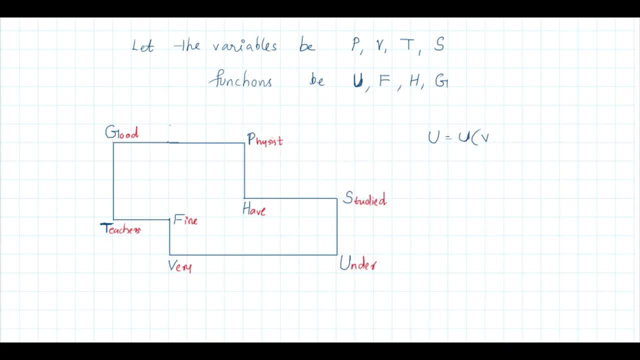 so I can write it as a function of v and s or I can write du as du. as this is a function of v and s means I can write dv and ds. dv and ds with respect to variation in v. there will be some change in u with respect to variation in s. 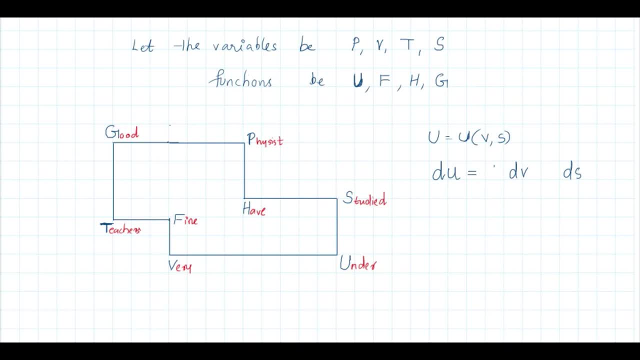 there will be some change in u now, since all these functions are having the dimension of energy. having the dimension of energy along with v, you have to write p. along with s, you have to write t- temperature, because p? dv has the dimension of energy, t ds has the dimension of energy. so 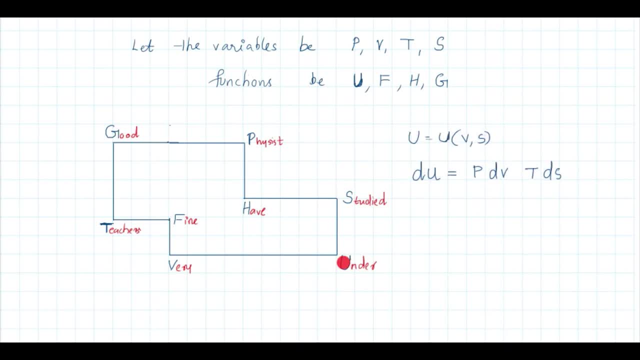 p, dv, t, ds. now we have to put sine: okay, whether it is plus or minus. for that- look at this figure again. in the case of u, s is towards top, okay, towards top and towards right, you have to put a positive sign. towards down or towards left, you have to put negative. 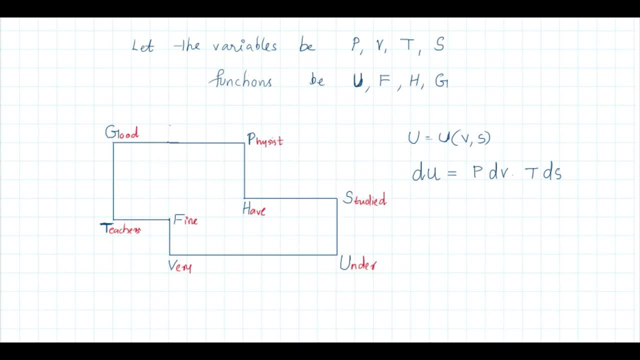 sign. since s is towards top, you have to put a plus sign for dds and for pdv. since v is towards left, you have to put a negative sign. so du is minus pdv, plus dds. in a similar manner, you can write dh, dh. what is dh? it is a function of s and p, because 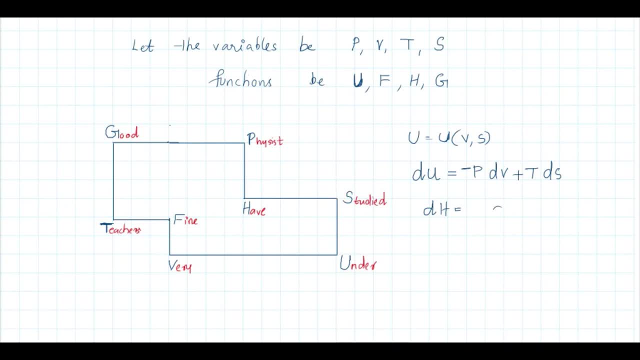 nearer to h, we have s and p, so dh, you can write it as ds and dp, ds and dp along with s. you, the only possibility is t along with t. the only possibility is v, dds, vdp. what about the sign? both are positive, because p is towards top, s is towards right. so both are positive. now, what about dg? what about dg? dg is. 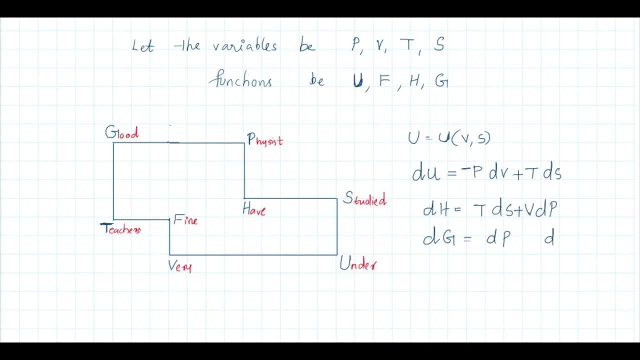 dp, then dt, p and t dp, dt along with t. we have v along with the t, we have s for t. it is downward. so you have to put a negative sign. p is toward right, it is positive. so the last one is df, helmholtz, free energy. it is nothing, but there will be a dv and dt. 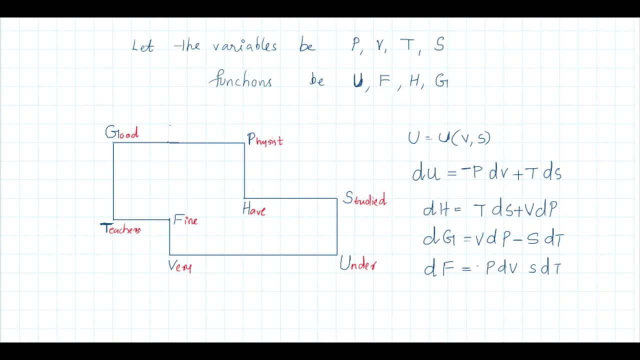 so sdt, pdv, both are negative because this is towards left, this is towards down. so this is the variation of various thermodynamic functions: u, h, d and f. then what is the relation of helmholtz, free energy, f? how can you find f? given you, if you give the internal energy, how can you learn f? you have to look. 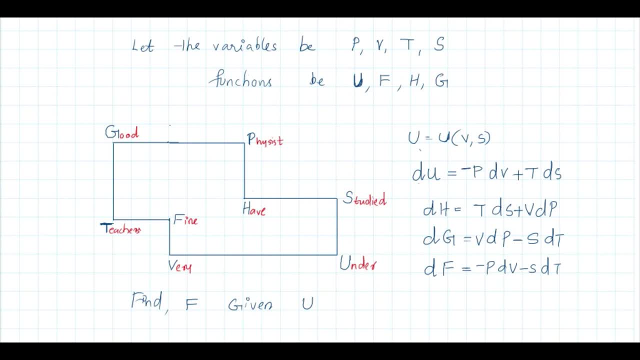 at the take u you have given u. u is a function of v and s. you are going to find. you are going to find f. f is a function of, u is a function of u. you are going to find. is that how you find f? f is a function of, f is a function of v and t. So f of vt given u of vs. So. 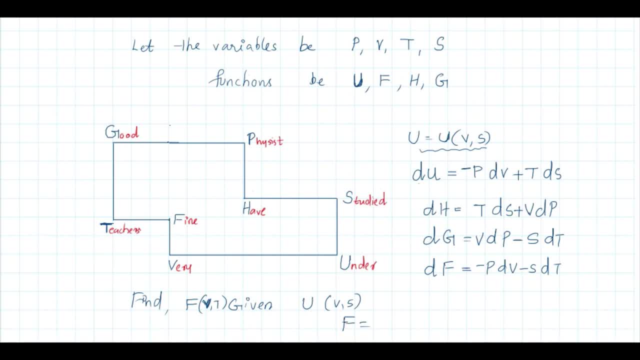 t is equal to f is equal to f is equal to u written there, u written. Then which variable has changed? See, v is here. v is here. Ok, v is common, But what came after t changed? 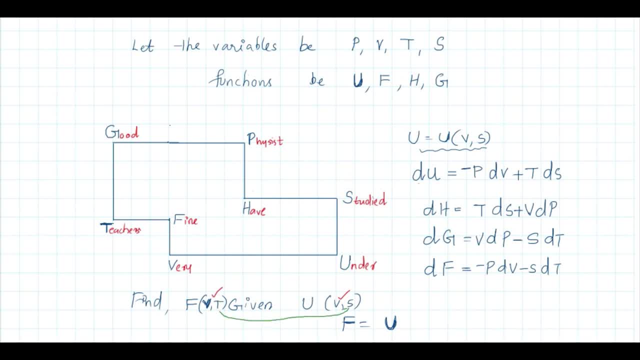 Variable t transformed to s. t transformed to s. So write ts here. write ts here. So f is equal to u, Then ts. Now you have to put a sign in between. How to put that sign? Go to v. sorry. 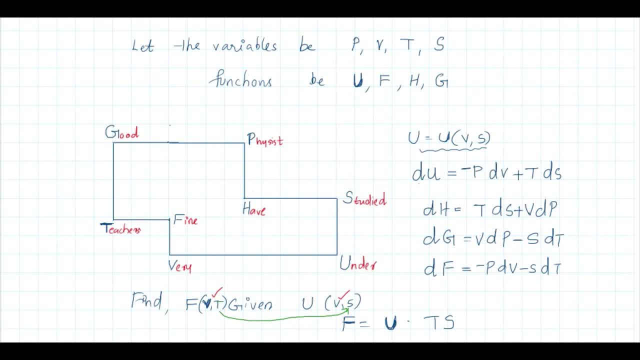 u. Where did we start? We started at u. Go to u See how s is written. The variable that changed here is s. Ok s changed to t. So see how s is written at u. It is in the top. 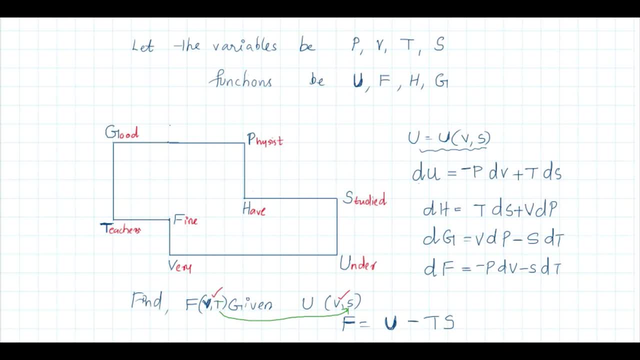 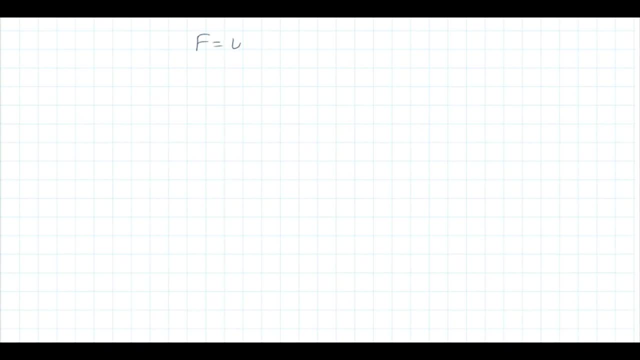 So it is positive. You have to put a negative sign. You have to put a negative sign. Ok, then f is equal to u. So f is equal to u minus ts. f is equal to u minus ts. We have to verify this. df is: 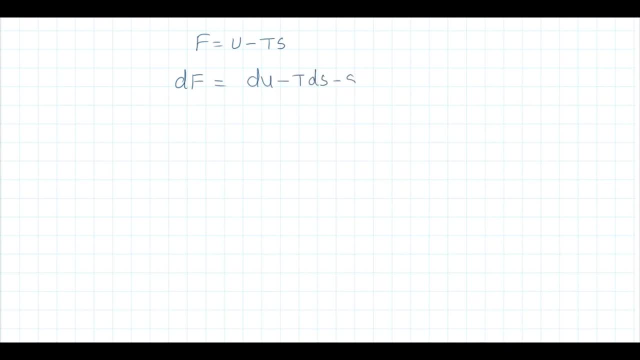 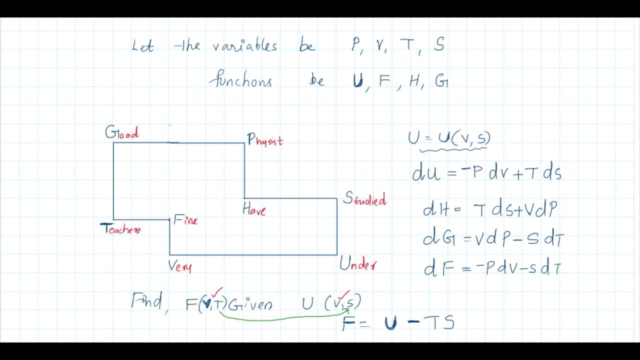 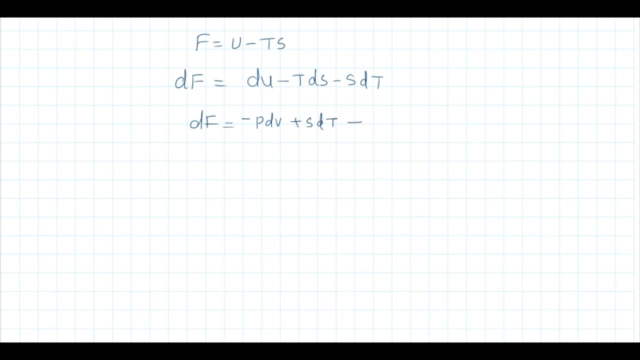 equal to du, minus tds, minus sdt. So df is equal to what is du. Du already know Du is. du is minus pdv, minus pdv, plus sdt, minus tds minus sdt. Then this sdt and sdt will. 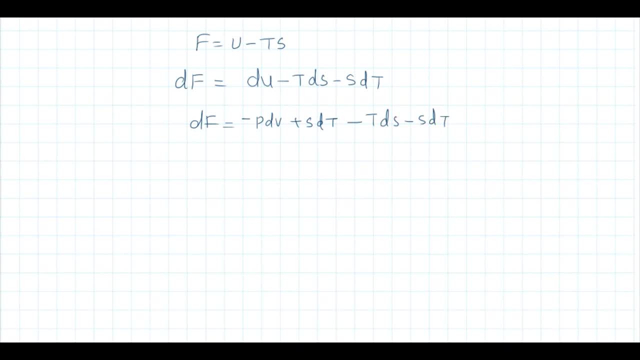 cancel This term and this term will cancel. So we will get df as minus pdv, minus tds. So it is the same as here, df. So this is the idea: f is equal to u minus ts, f is equal to u. 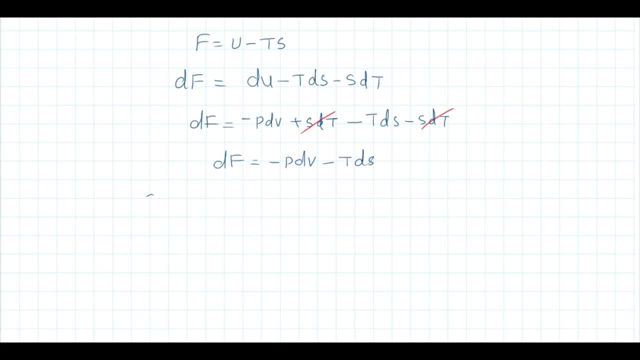 minus ts. Then what is g Given given f, find g, Then we have to find g. So we have to find g Given, given f, find g. F is a function of, or again, f is a function of b, and 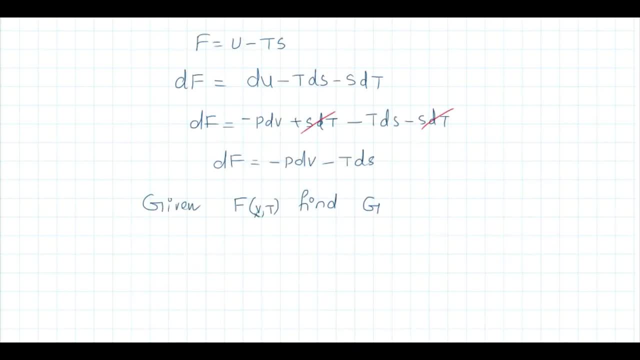 t. F is a function of b and t. g is a function of g is a function of b and t. Then we can write: g is equal to g is equal to f. Here which variable can change t? one of both? 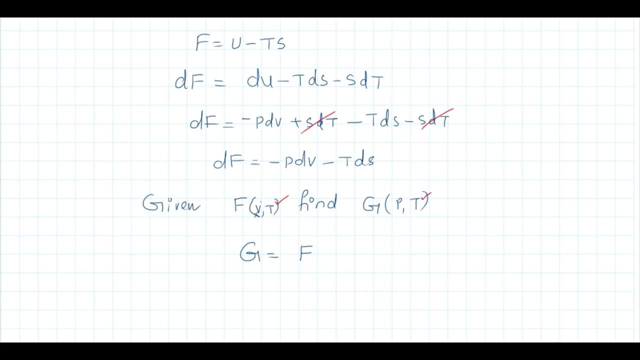 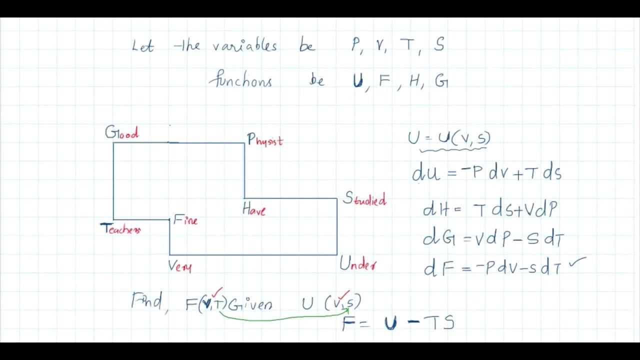 is the fixed. What are the variables that can change? Who are the variables that can change? So V changed to P, Then you have to write a PV here. You have to write a PV here. Now the remaining thing is to put a sign. 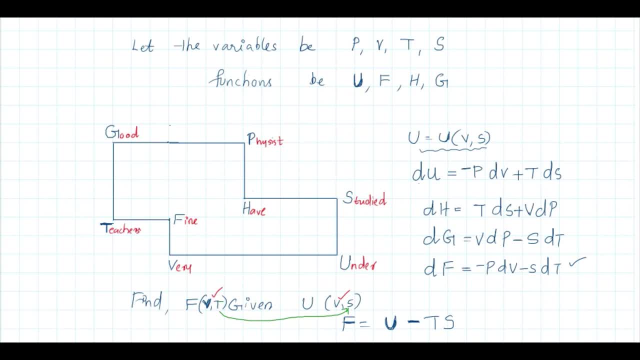 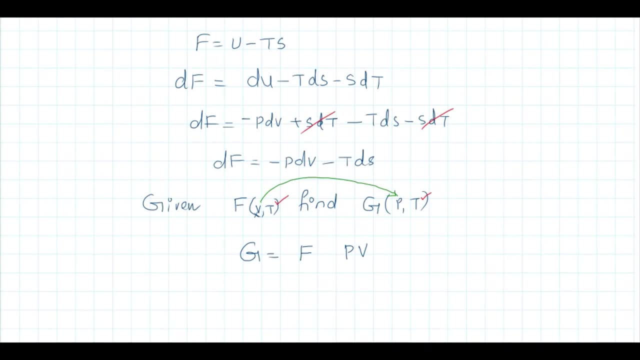 To put a sign For that. go to V. Go to V. this volume In F in Helmholtz, free energy, V is towards downward. Okay, V is downward. That is what changes here. That is why there is an opposite sign. 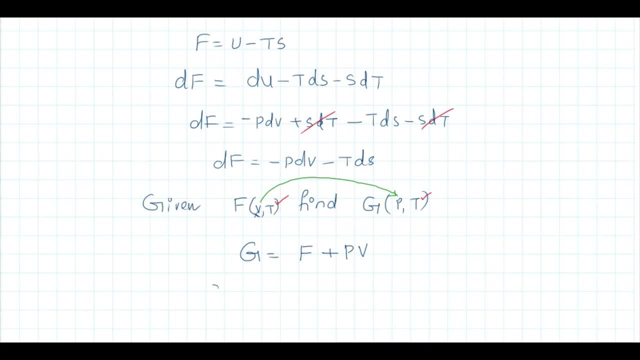 Plus, Okay, V is like this: V's sign is negative when it is downward And the opposite sign is to be put here, But only when you write DG, DFL, DFL, DFL, PDV is negative. Now PDV can be cancelled. 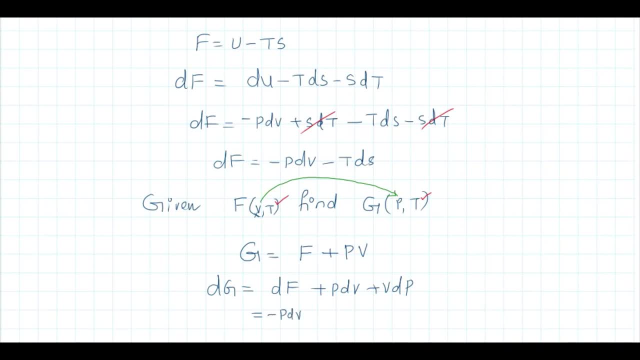 DFL. you know, DFL is minus PDV, minus EDS. Plus, here is a PDV plus VDP In this. PDV cancels This PDV cancels because It is because you put a plus, If you put a minus here, if you put a minus, PDV will not cancel. 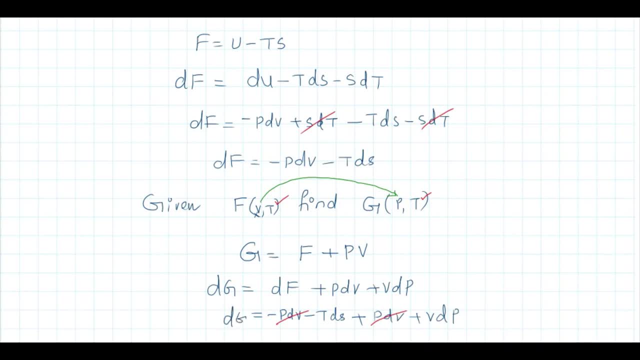 You won't get DG correctly. So here we are putting plus and minus. Whichever variable changes, that variable is already a function. If it is positive, there is a negative sign. If it is negative, there is a positive sign. 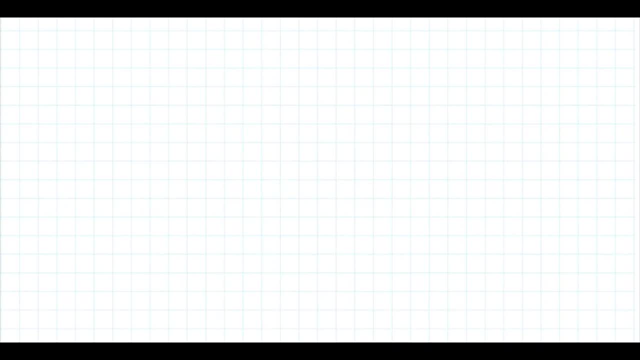 So we got an expression for G: It's free energy. Similarily, we can find H. If you have a knowledge of U, you can find any thermodynamic potentials. Using this idea, you can find any thermodynamic potentials or thermodynamic functions. 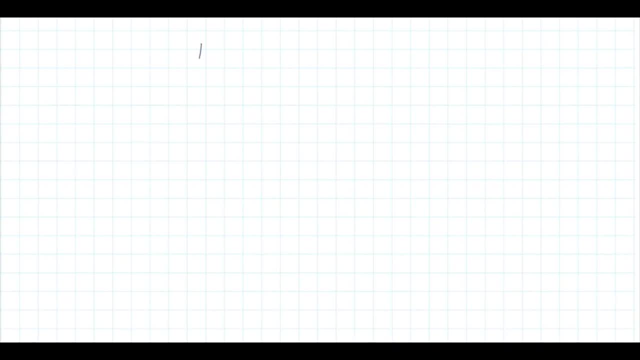 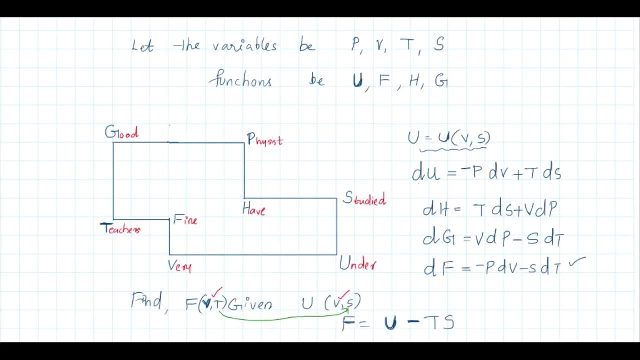 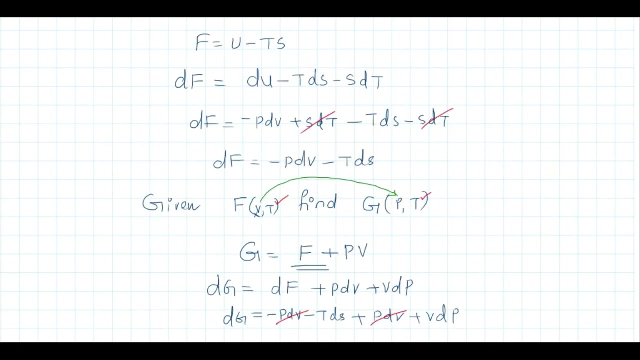 What is H in terms of F, H and F? H is here, F is here, H is a function of S and P. F is a function of T and V. Both the variables are changed. The variables in H are P and S. Since both the variables are changed, you have to write. 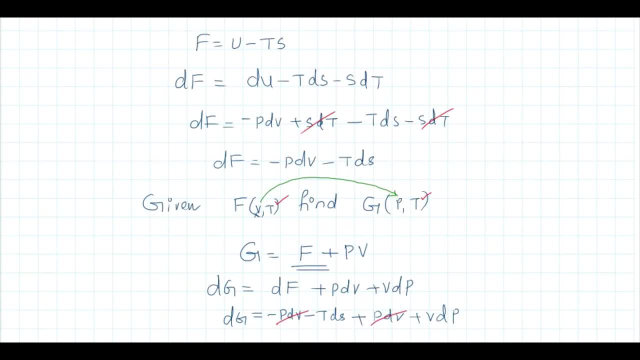 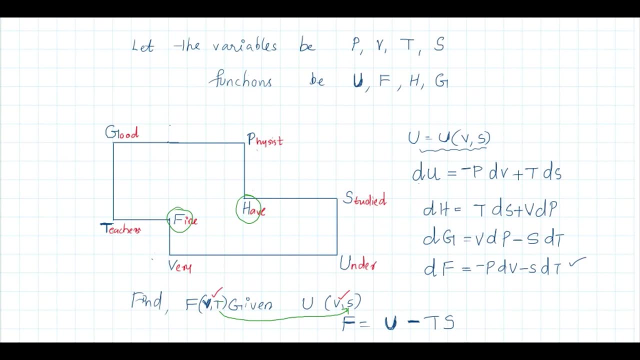 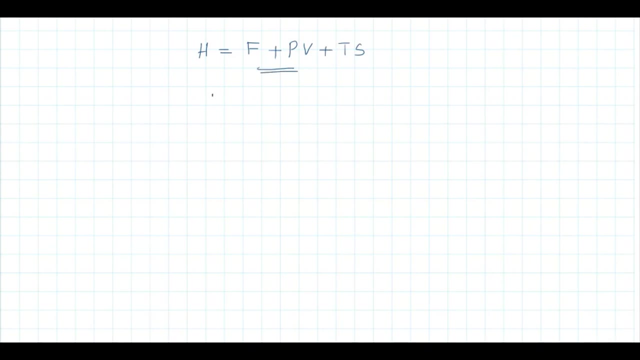 PV as well as TS. Now the rest is to put a sign In F. both V and T is negative, So you have to put a positive sign. This is the relation for H in terms of Helmholtz free energy or F plus PV. What is F plus PV? 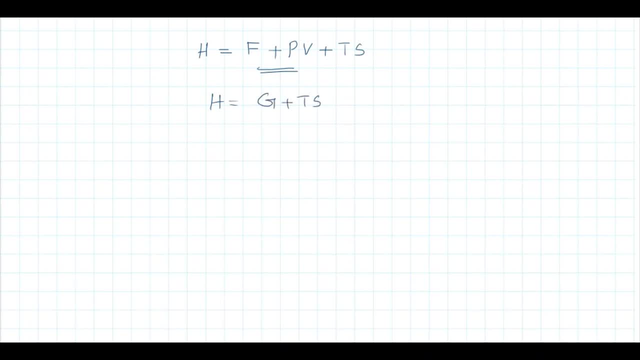 It is Gibbs free energy. So you can write it as: H is equal to G plus TS, H is equal to G plus TS. I hope all the functions are written. Rest of them you can write in a similar manner. So once you have enthalpy and internal energy. 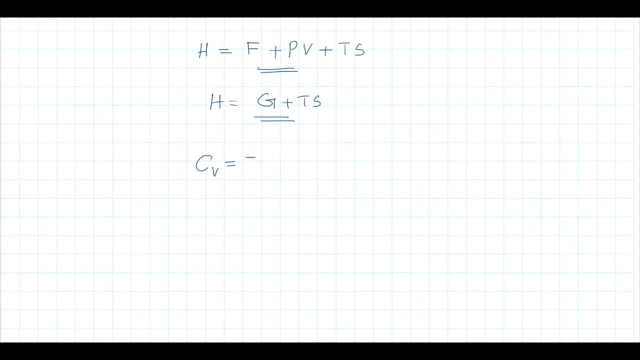 you can write specific heat up as a constant volume, which is T dou S by dou T At constant N and V, and that is nothing but dou U by dou T. Dou U by dou T is the constant. Where U is the energy Earlier, we used the symbol E.